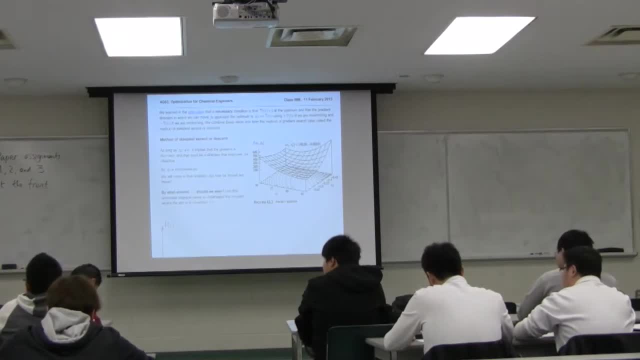 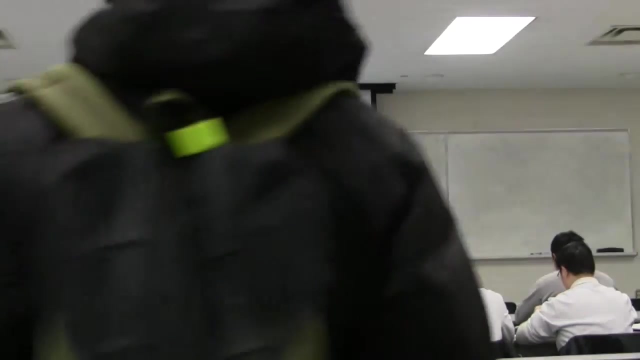 decided to modify a little bit of what I was going to talk about on the last page of the prior handout, So the best option is actually just to ignore the last page of 6A and we'll just keep going here with 6B. The reason why I wanted to do that is because in the prior 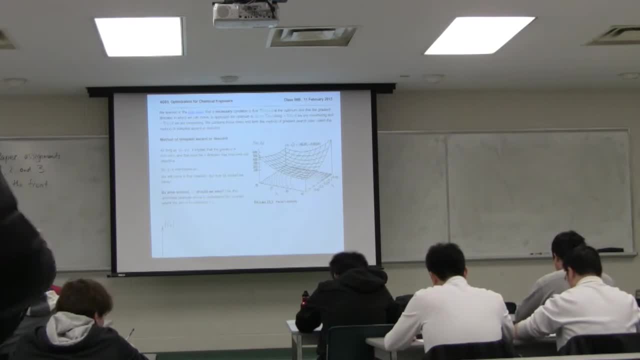 handout. I'd planned to go straight to the multidimensional visualization, But when reviewing this again over the week, I've been thinking that it might be better just to step back and take a look at it univariately first and then step up to the multivariate case. 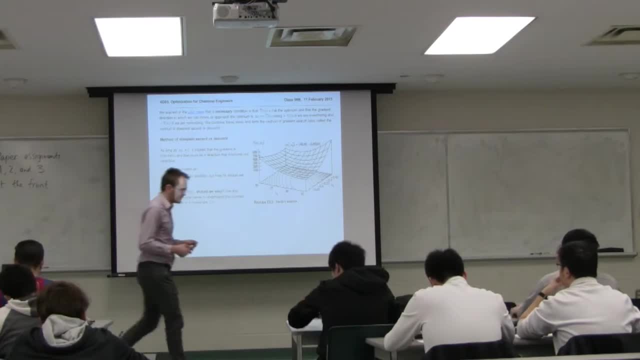 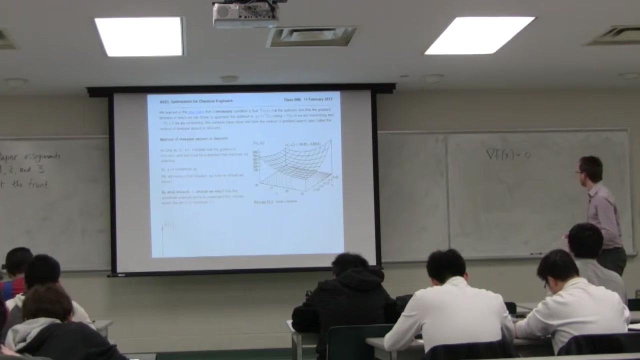 So let's get started. So let's do that then. And basically we established two things in the class last Monday. The first is that condition right up there that delta f of x must be 0 at the optimum, And that's the multidimensional expression. The univariate version of that is that f dash. 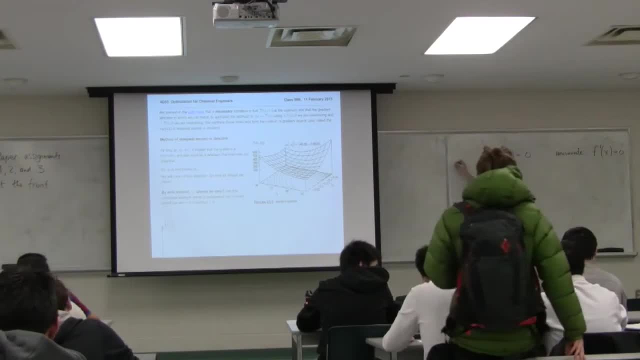 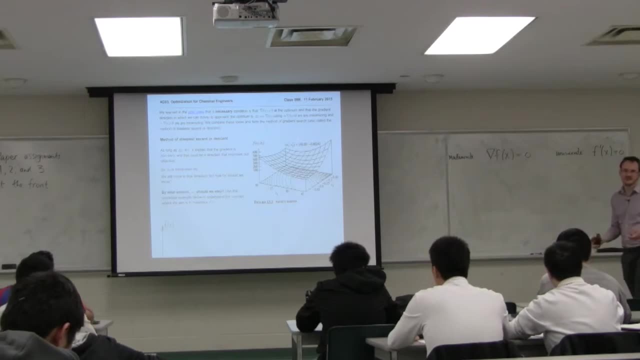 of x must equal 0.. So this is the multivariate Statement and that's the univariate statement, And they really are the same thing. This is more specific, though here for the multivariate. This is saying here: this is the partial derivatives. 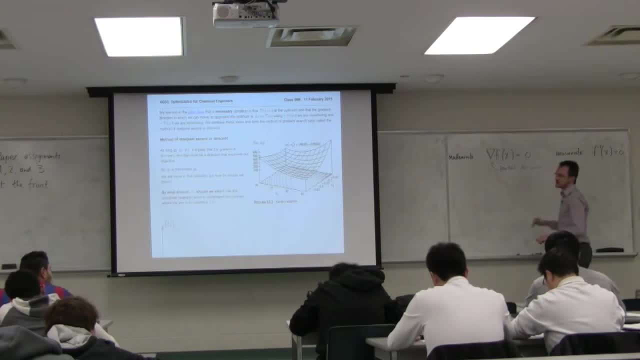 OK, so that is what we call our necessary condition in the class last week. Then we know that that characterizes when we're at the optimum. So you might want to emphasize this: This is at the optimum, OK, so that's a good way to know that you're there. 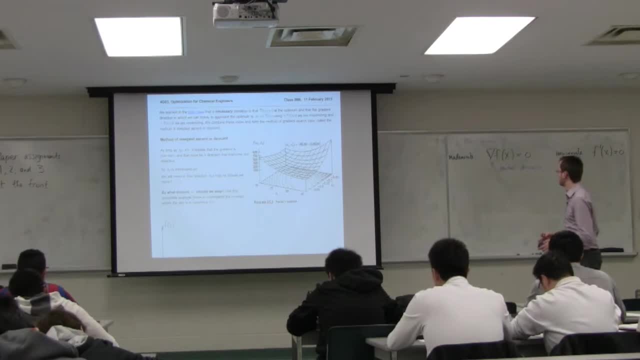 But we're not there. whenever we start the optimization problem, We're going to be away from the optimum. So we want to move towards the optimum And we established last class that the way to do that is to climb this direction of steepest. 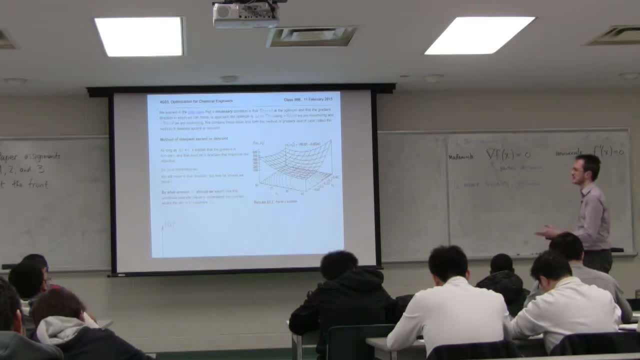 strangest: ascent or ascent And or, if you're looking at minimizing to look in the direction of steepest descent, So that move that you make is equal to delta x. I should say this is your move direction we're going to talk about. 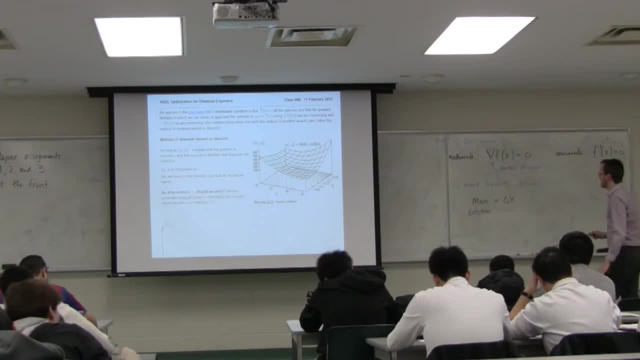 the actual move that you make. the move direction is delta x and is equal to plus or minus. this gradient direction And the plus or minus up front here depends on if you're maximizing, and if you're minimizing that would be negative. 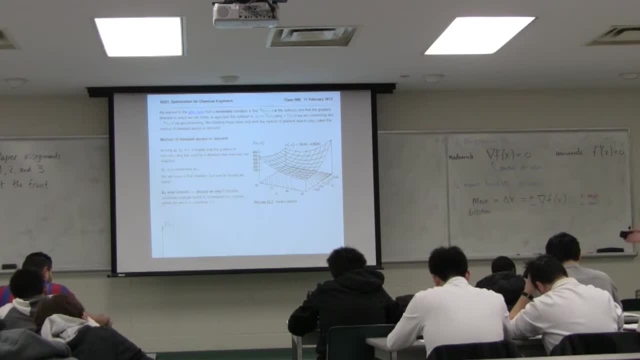 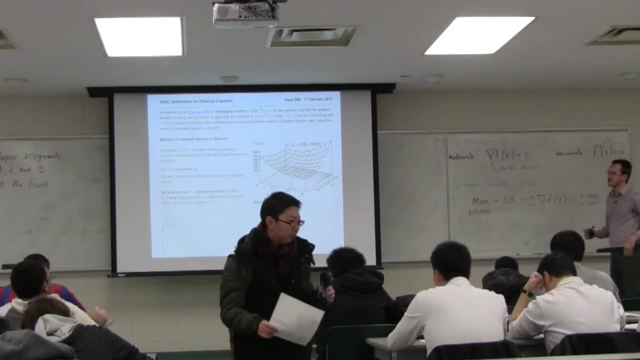 So your move direction? that is just a compact statement of saying: go up the mountain, up the gradient if you're maximizing, go opposite to the gradient, negative to the gradient if you're minimizing. So we're comfortable with interpreting that over there. 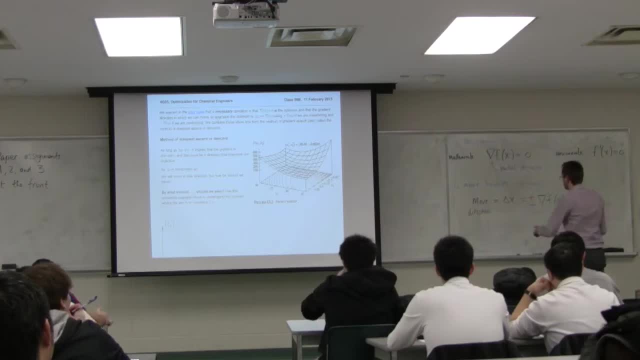 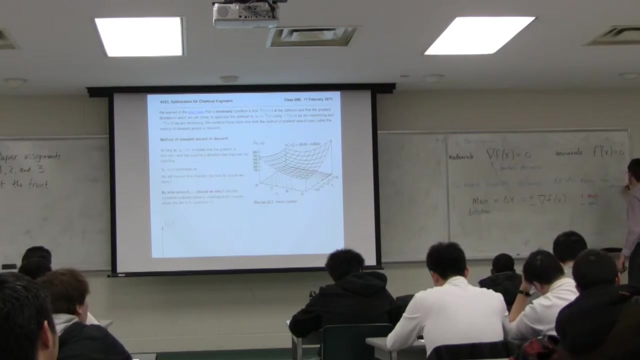 And this move direction is going to be non-zero if you're not at the optimum. So delta x is non-zero away from the optimum. So the interpretation of that is: as long as delta x, that move direction, is non-zero, you've not reached an optimum yet. 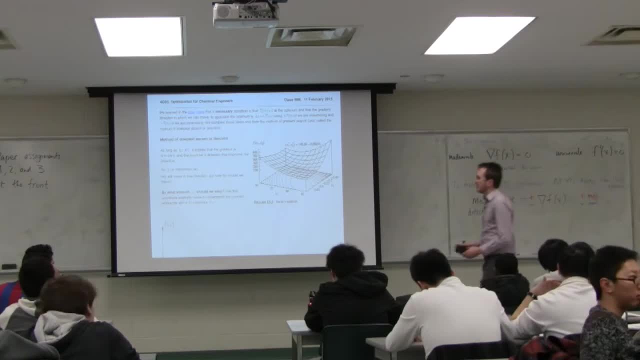 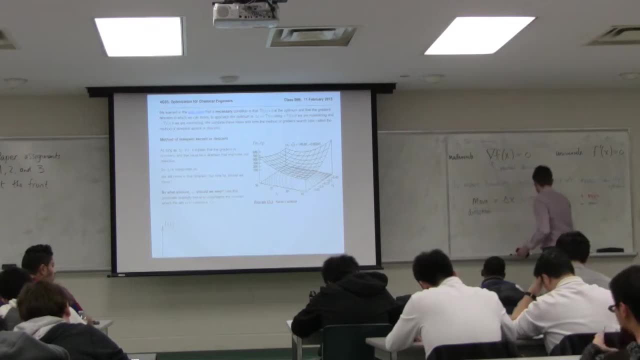 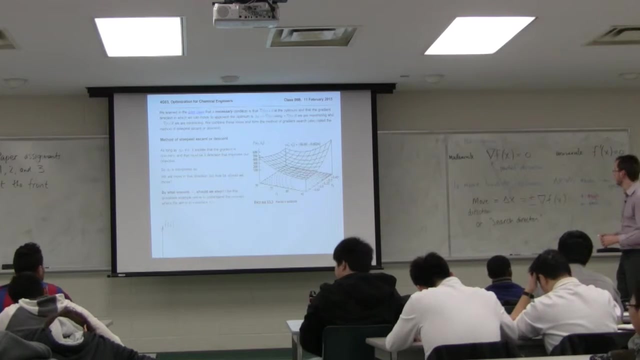 and you need to keep going. Now, delta x. The key interpretation of that is it's your move direction, or your search direction, as it's sometimes called, Move direction or search direction. But the step where we left this in the class 6A on Monday. 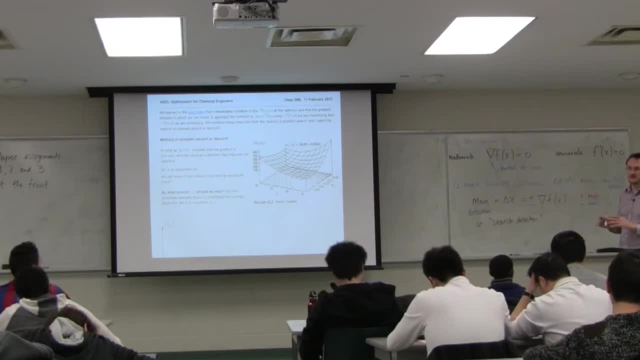 was. we know that that's the direction we need to go. The optimizer is telling you: go that way, but we don't know how far along to go Right. So imagine if you were up here at this point. The optimizer knows to head down. 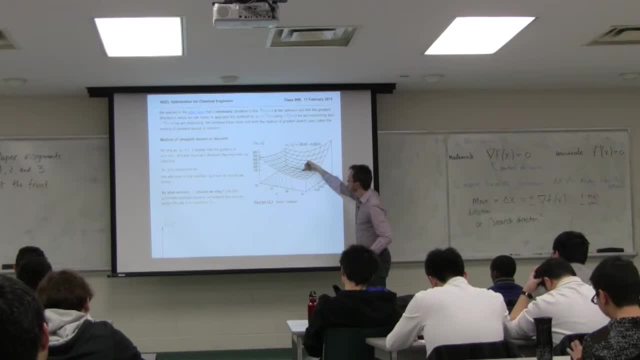 but it doesn't know how far down Right There's a certain amount that you move down where. that's great. but if you had to keep going you'd start to go up that bowl again. So you can't just say: head in that direction. 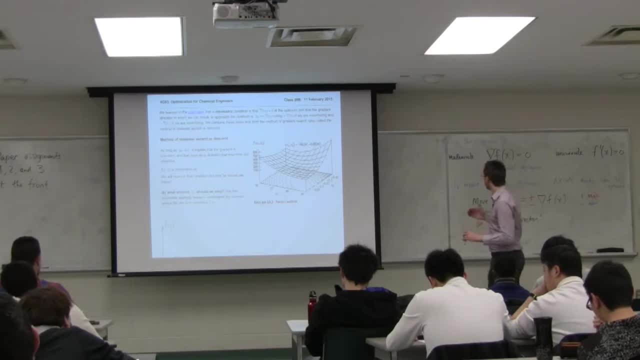 You need to say by how much, And we try to go only as far as necessary so that we don't bypass or exceed the optimum goal that we're trying to look for. OK, Now, to emphasize this, let's look at a univariate picture. 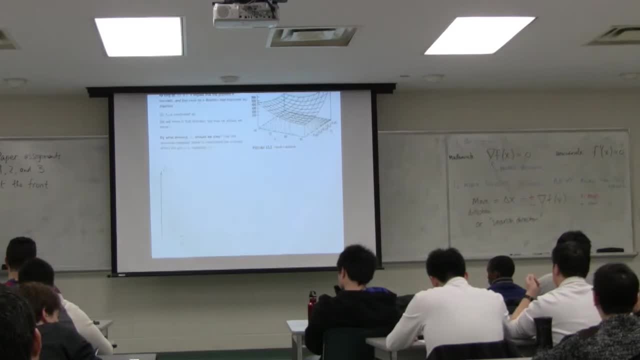 And I've drawn the starting point over here And we'll add to this diagram Because I want you to have this in the mindset of the computer code. The computer code does not have that geometric picture. I've emphasized this many times in the class. 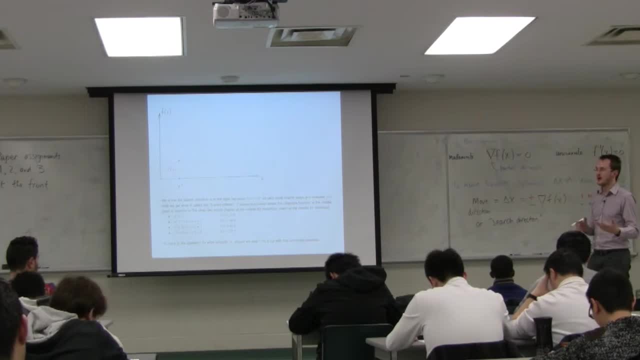 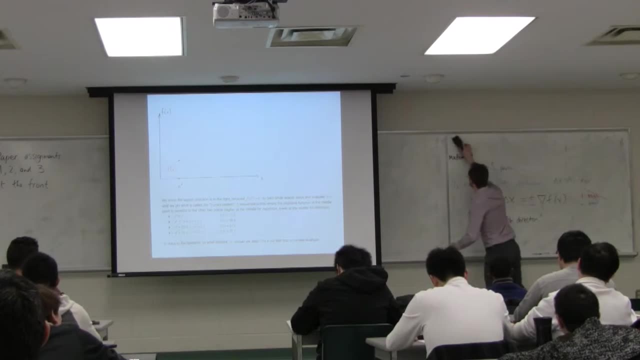 The computer software does not see a geometric view of it. We like to learn about it geometrically, But let's take a look at how a computer algorithm then would proceed in the simplest of cases, the univariate case, And it's fairly intuitive. what's going on here? 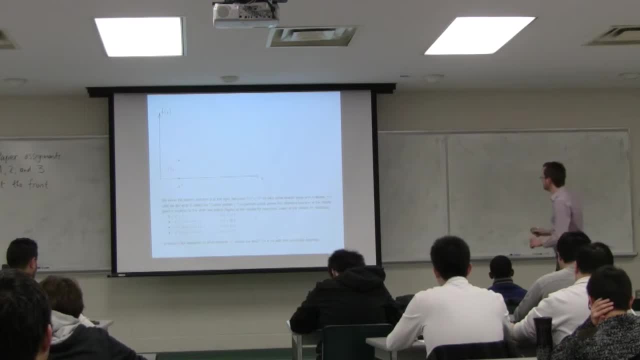 And then we'll scale it up to the multivariate case. So in the univariate case we have a single variable, x, that we're trying to move, And our current estimate, or our starting point then is some x0.. 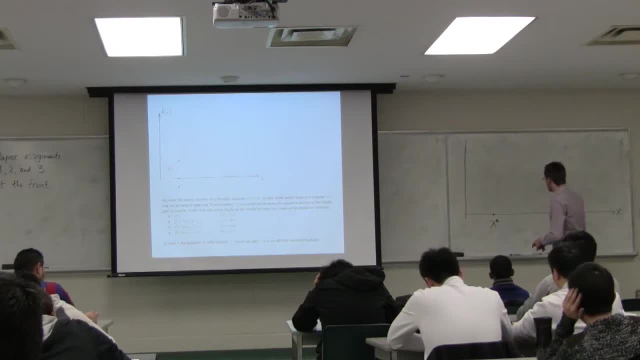 So that's my initial condition over there And the function can be evaluated at that point. So I can go find this f of x at that particular location And I can also go find the first derivative of that function And at that point the first derivative of the function. 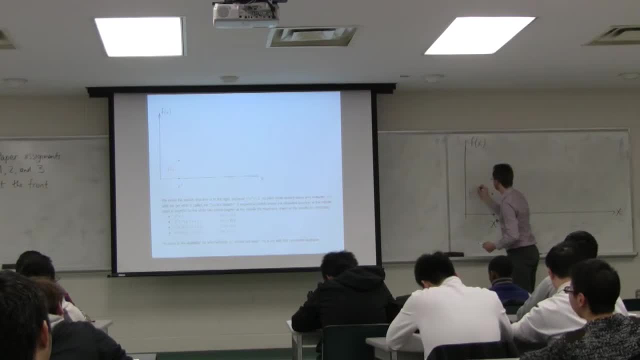 is given by that red line, f dash of x, And it's particularly at f dash of x. So that's f dash of x0.. So all we get is a local estimate of the slope. Now I've been told this is politically incorrect analogy. 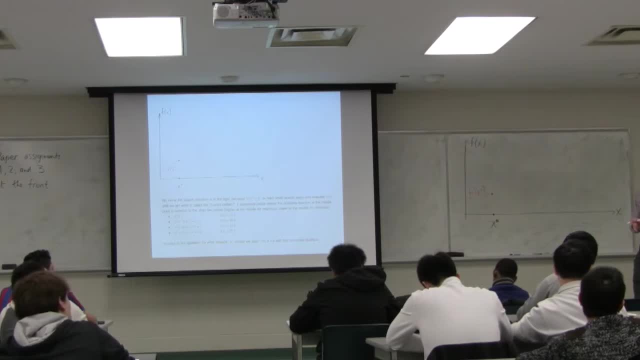 to use, but I think it's still descriptive. Imagine that you're a blind person at that point And what this is doing is you want to climb up the mountain. Now you cannot see what's around you. We don't know what this function f of x looks like. 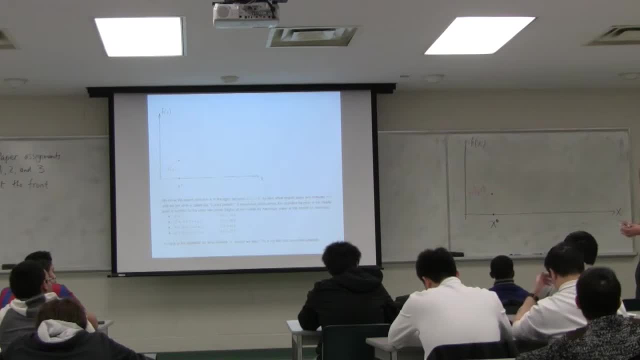 You're totally in. that's invisible to you. What you can do is you can touch the ground with your cane or your stick and you can feel which direction the ground is most going up in, And you would proceed if you want to climb the mountain fastest, to go in the steepest direction. 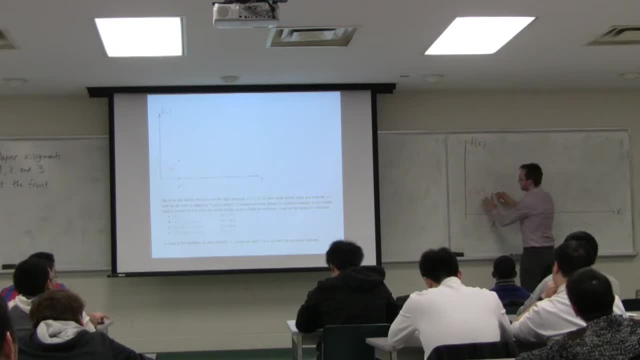 So this f dash of x is a geometric way of saying: go up the mountain. How far of a step do you take? Do you take one big step or do you take several smaller steps and keep climbing up? OK, So this is the analogy. 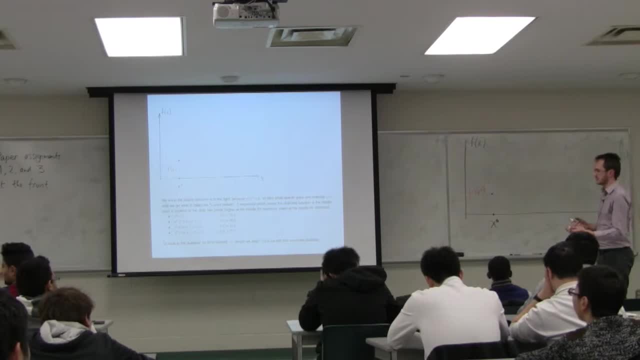 Now there's many algorithms to do this stepping and there's not one single right way of doing it. So one way that you can do is simply to say: well, I'm here, I'm going to take some sort of step by an amount. alpha. 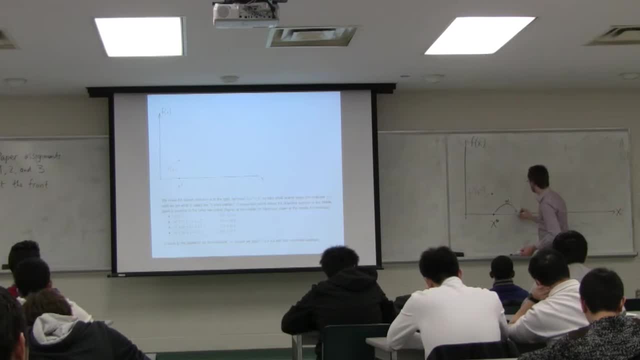 And then I'm going to evaluate that function at that point And so at that point I get the value of f At that location And you can take another step, 2, alpha, And you can find the function is over here now. 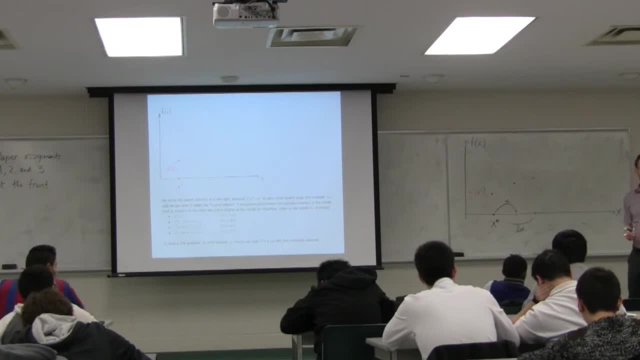 You don't find the slope at that point. No, we're not calculating the slopes, We're simply evaluating the function. And I can take a third step, 3 alpha, OK, OK, OK, And I can evaluate the function at that point. 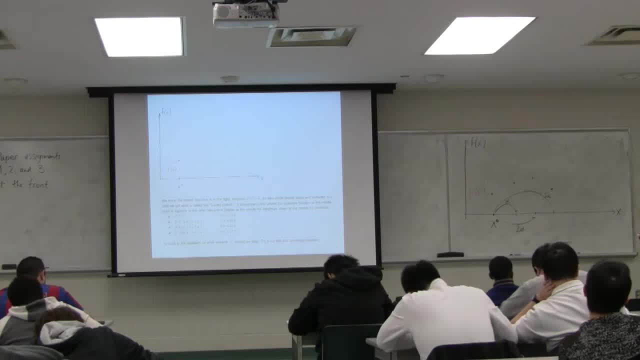 So you've taken three additional steps: alpha, 2, alpha, 3, alpha- And you already can start to guess where this might go. You can start to build a local model, a local approximation of what this function f is doing. We don't know what's happening in between these points. 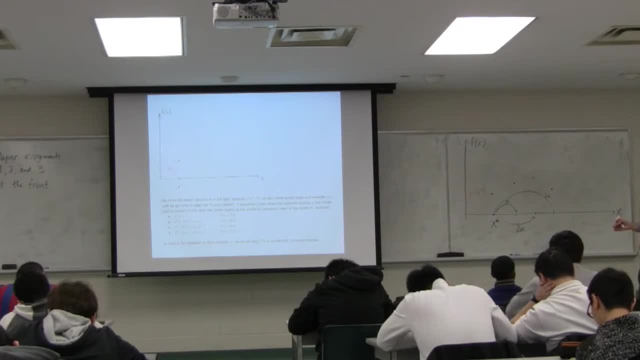 But. But for the most part, most functions behave fairly well, So we can expect that there's some sort of continuity and smoothness there. Now what we will go do is: our goal is to approximate that function, And one of the easiest ways to approximate a function. 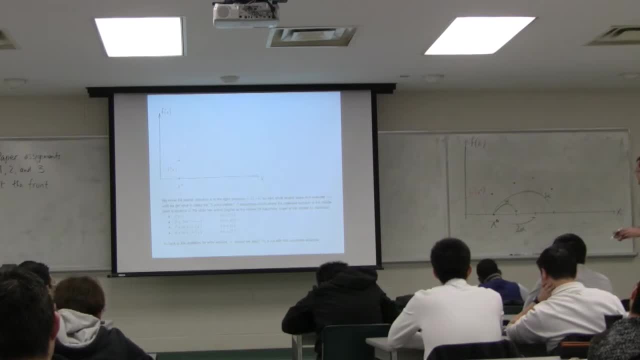 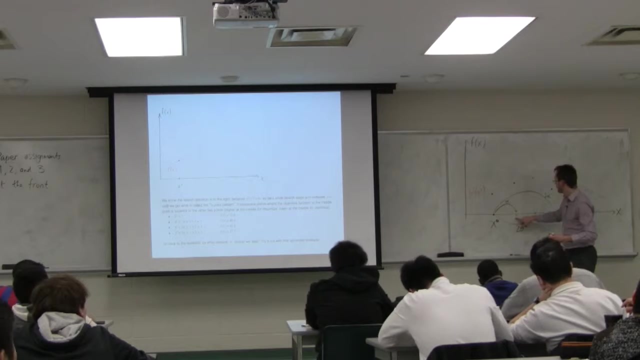 is to build a quadratic approximation for it. So what we can do is we can use any three points here to build a quadratic approximation. I could use any three points here: x0,, 2 alpha and 3 alpha. Or I could use this point here at 1 alpha, 2 alpha and 3 alpha. 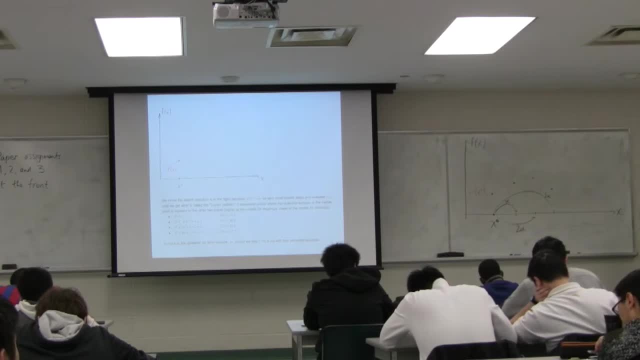 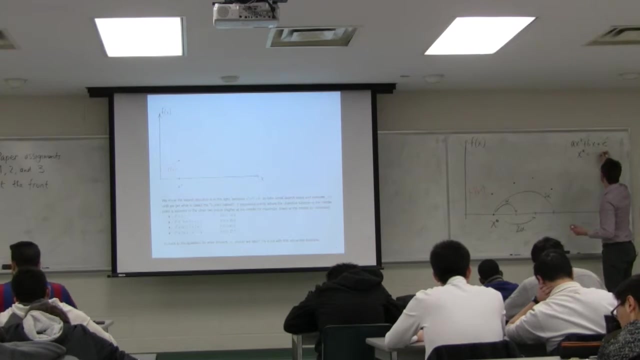 away from x0. Any three points can be chosen to build a quadratic model. And then we go to find we know that the equation of a quadratic is ax squared plus bx plus c, And we know that the optimum of a quadratic is minus 2b over a. 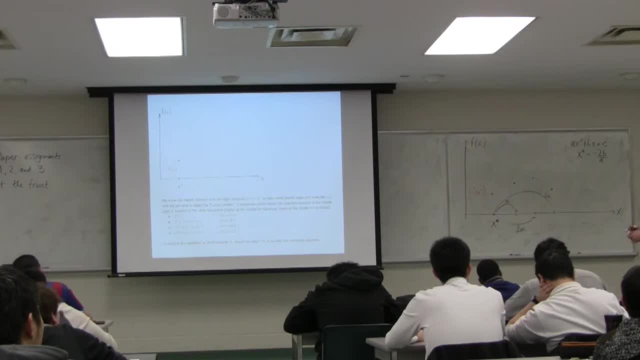 I think off the top of my head, I might be a little bit wrong, But any quadratic can be uniquely found: the peak, the location of x, which maximizes or minimizes that quadratic. All we need, though, is three points. 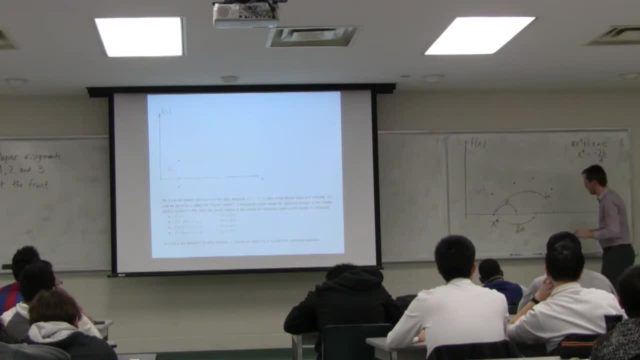 But we don't need any three points. There's a special requirement that these three points must have. Let me illustrate it this way: for example, If I gave you these three points, could you fit a quadratic to it? You can fit a quadratic to any three points. 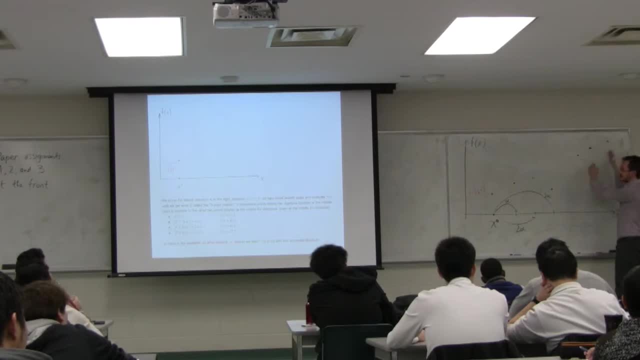 But the quadratic is not going to turn in these three points. The quadratic might fit over there And the turning point's going to be outside the three points. Similarly, if I gave you three descending points again, you could find the quadratic. 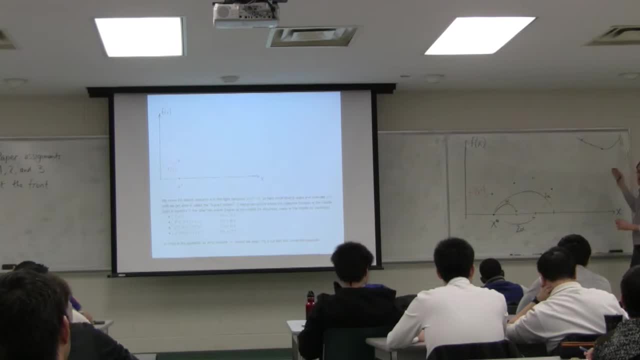 But the quadratic is going to go through those three points and turn outside the three. There's a special requirement: is that the three points must have this sort of behavior, That if you're trying to maximize, the middle point must be greater than the other two. 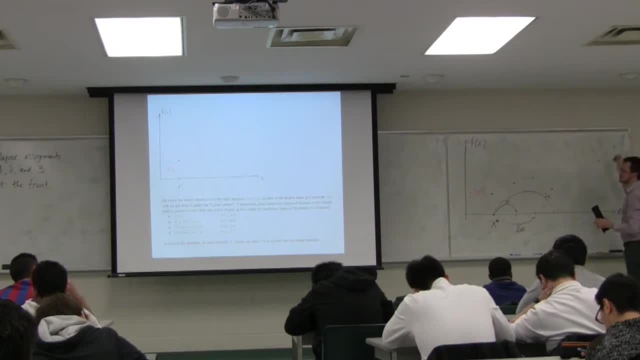 And if you're trying to minimize, the middle point must be lower than the outer two. So we call that any three-point pattern. We want a three-point pattern, three sequential points where the objective function in the middle is superior And the objective function in the outer two is lower than the value. 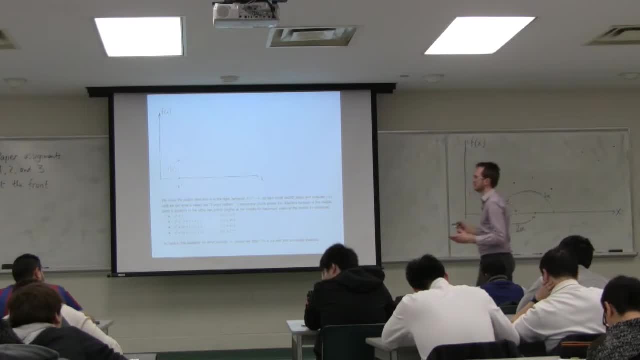 at the outer two points And I've intentionally left superior there because you want that to be higher for maximizing And you want the middle point to be lower when you're minimizing. So as long as you can get any three points that follow that pattern, you can fit a quadratic. 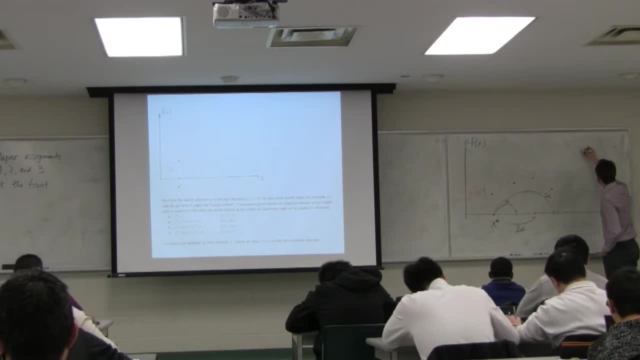 And that quadratic will guarantee to turn around inside that range. So they're my three points. The quadratic will turn inside the lower and the upper points, And that's what we're going to do. So we're going to do that, And then we're going to do that. 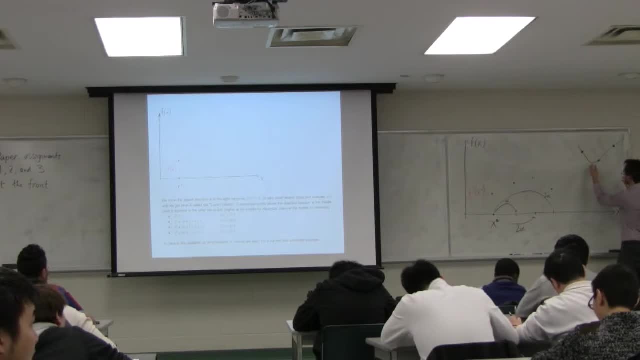 And then we're going to do that, And it might be that the turn is between one and two, It might be that the turn is between two and three, Or it might be that the turn is exactly at that middle point, if it's coincidental that way. 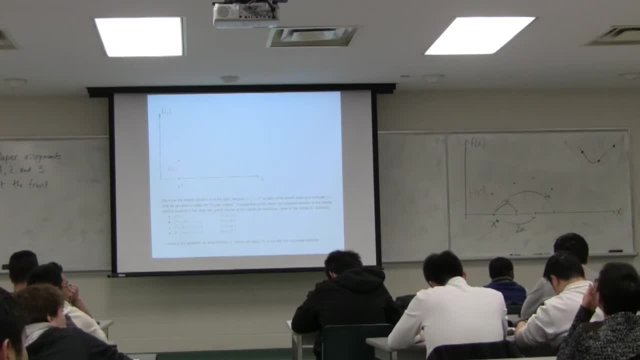 Is there a reason why we use quadratic Like? is there not an opportunity that it could be a linear relationship? It could be a linear relationship, But a linear function can't be optimized. A linear function, A linear function, just keeps going up and up. 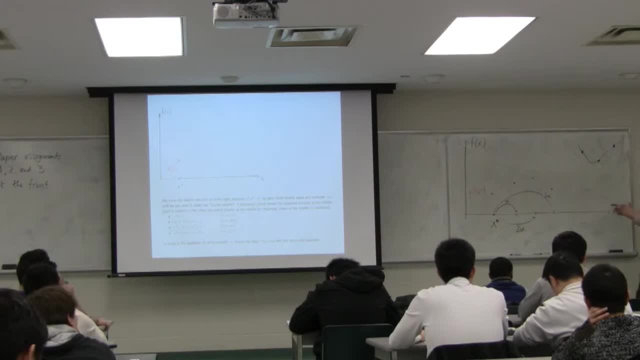 Oh yeah, Unless if it's unbounded. Yeah, But what we're going to do is we're going to keep stepping by alpha 1, alpha 2 units, alpha 3 units, until we find a three-point pattern, Any function that has an optimum. 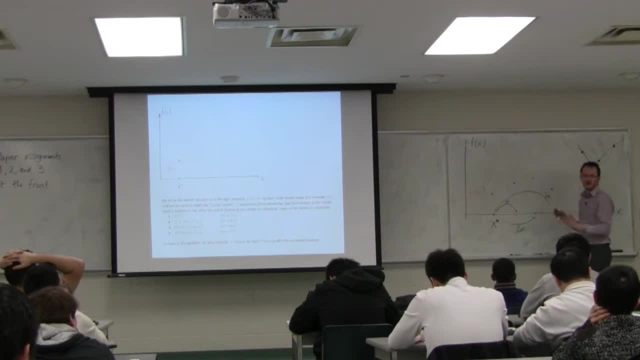 if you keep stepping with this, you will go up and then start to go down again, Unless no optimum exists. Then you'll find it with just your steps. You just keep stepping and stepping And the algorithm will have to do that. You'll have to terminate because there's 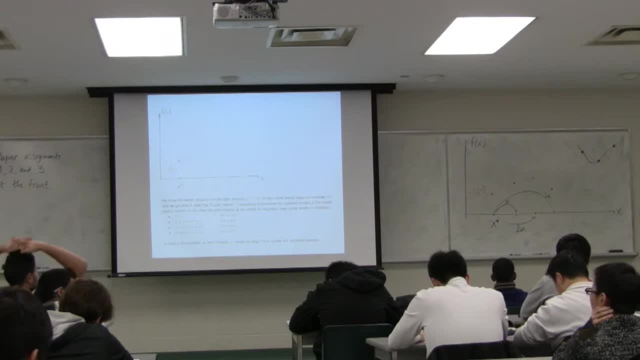 no actual optimum in that range. So, as you keep making steps to find the three-point pattern, does your x, like your actual x point that you're looking at, change with the three-point? No, No. So what we're going to do here is: I'm still at x0.. 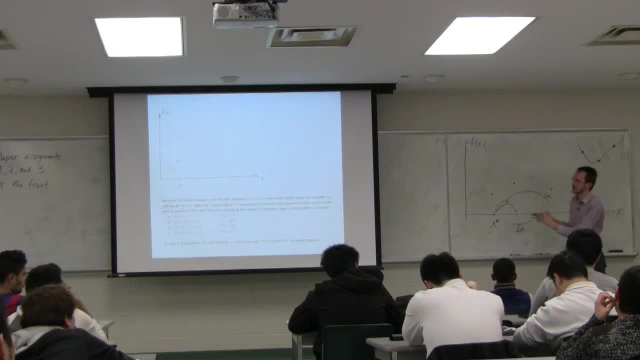 What I'm doing is I'm essentially finding how far to step right. Coming back to my problem, This is the problem in today's lecture: How big of a step do you take? We know which direction to go in. We just don't know by how much. 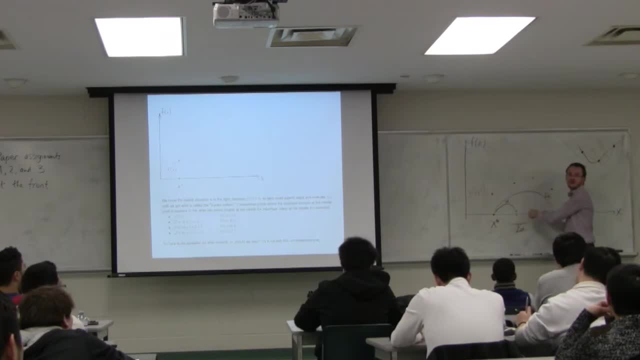 So I'm going to place my x1 wherever I find this mini-optimum here, So I'm solving this smaller problem. Then I'm going to place x1, repeat: find x2.. OK, So how we find a three-point pattern can be fairly flexible. 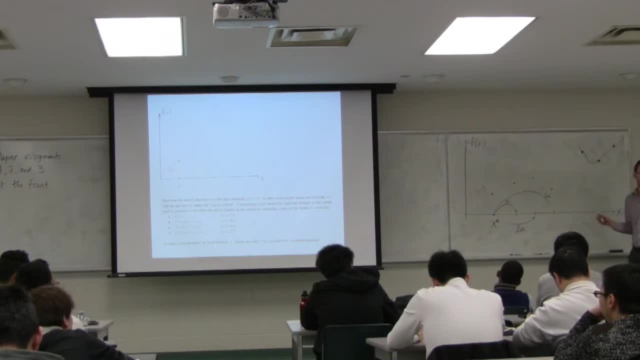 Here I'm stepping in steps of alpha 2, alpha 3, alpha, 4, alpha. Some algorithms go as follows. They say: step by alpha 2, alpha, 4, alpha, 8, alpha, 16, alpha And you can code up whatever exotic strategy you like. 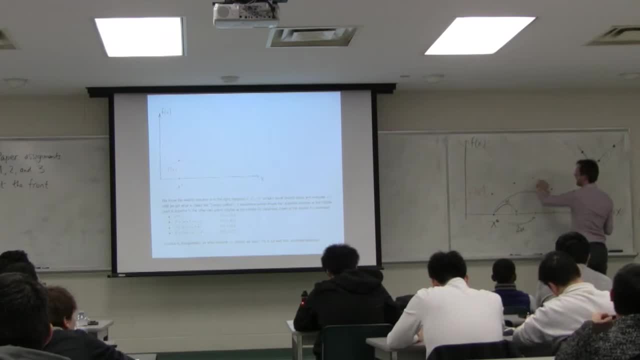 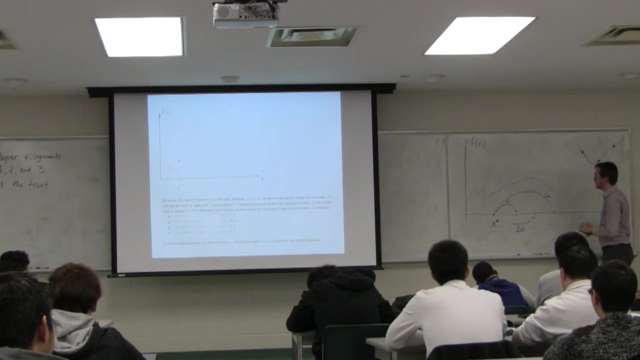 It doesn't really matter, as long as you find any three points that approximate that function. So let's perhaps draw the following here In blue: I'm going to draw the true function, OK, And if I use these three points over here? 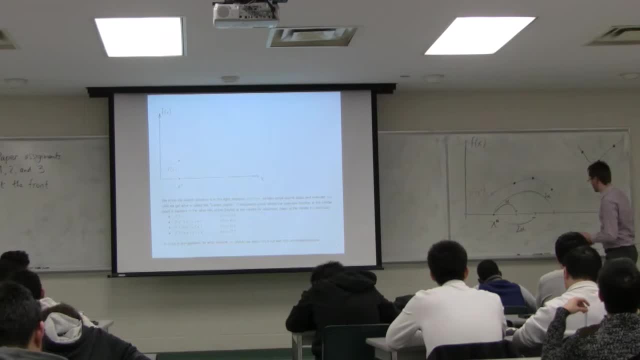 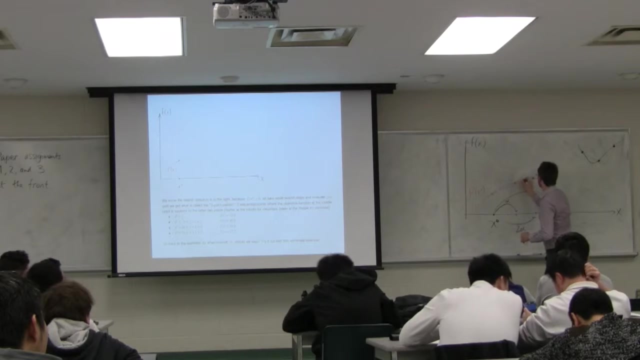 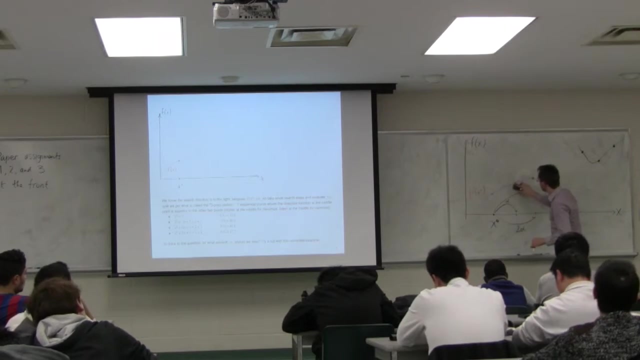 what I'm essentially doing is I'm fitting a quadratic through those points And it might be. let's draw this quadratic then in dashed red. That's not quadratic. eh, OK, that's probably a little bit better. The key point is that when you fit that quadratic, 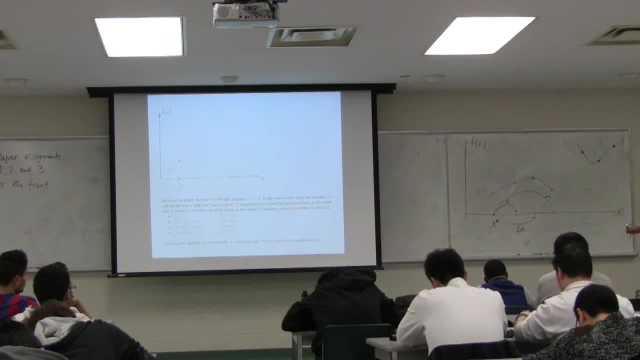 to those three points. the quadratic passes through the three points that you've selected And then we can go solve that problem- ax squared plus bx plus c- and find this location as my optimum to that quadratic. Then what we will do is just: let's clean up here a bit. 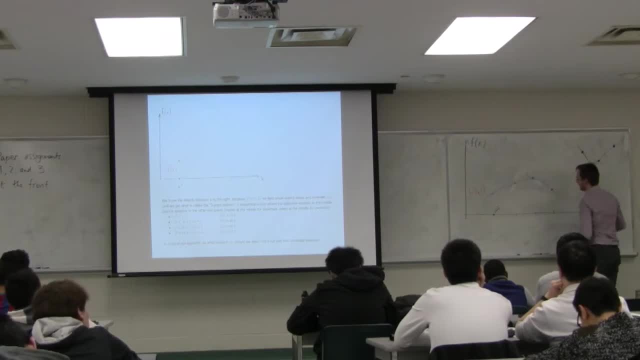 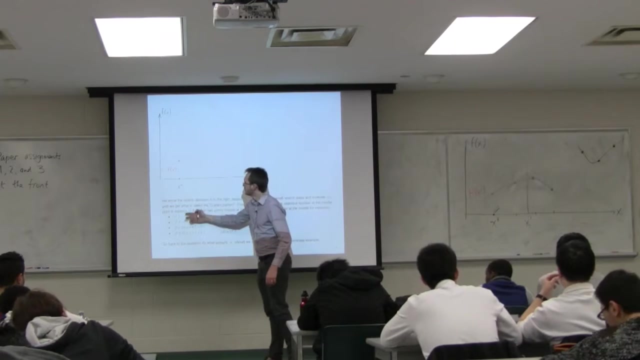 is. on my next iteration, I'm going to set that location here as x1. And I'm going to repeat this process of hunting for the optimum. So let's take a look at how we can optimize this. Here is an example where, at x0, which 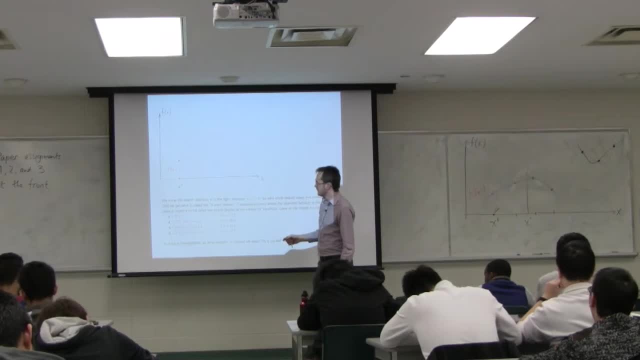 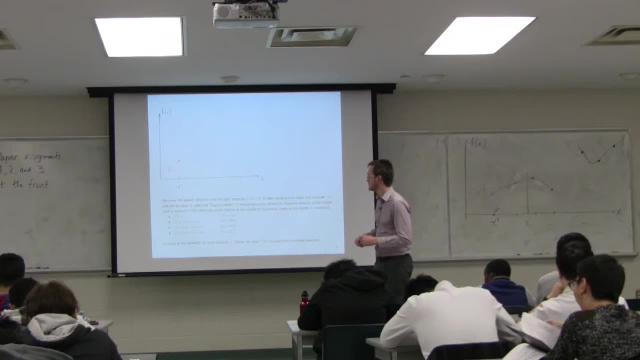 I've specified here at the point 1, let's step by alpha. I'm choosing alpha to be one unit, two units, three units- Again, that's arbitrary, That's up to the user to specify, or the algorithm to specify what these guesses are. 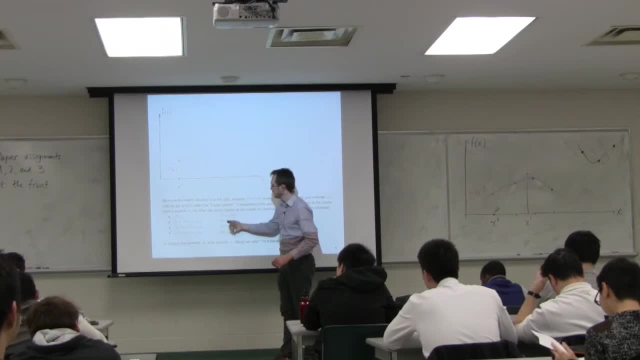 And we evaluate the function at these points: f1, f2, f3, f4.. When we see that, we notice that we can have a three-point pattern here. f2 is lower than f3.. f1 is lower than f3.. f2 is lower than f3.. f1 is lower than f2.. f1 is lower than f2.. And f2 is lower than f3.. And f1 is lower than f2.. And f2 is lower than f3.. 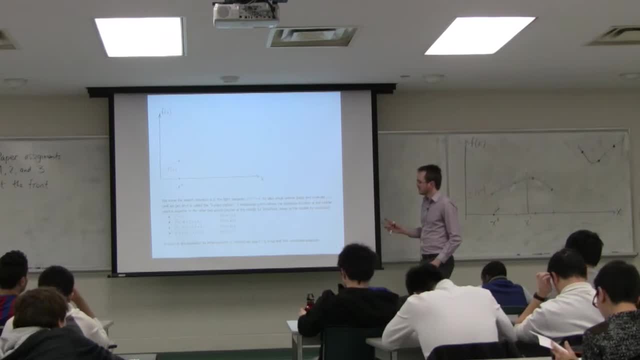 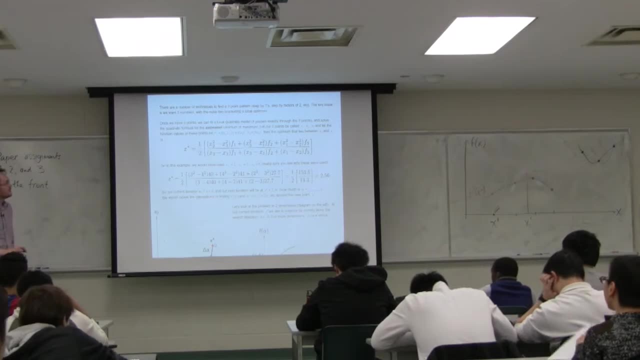 f1 is lower than f3.. and f2 is lower than f2.. f4 is lower than f3. So we can fit the three-point model to that And what we have, and there's no need to derive this mathematically. but if you give three function values, 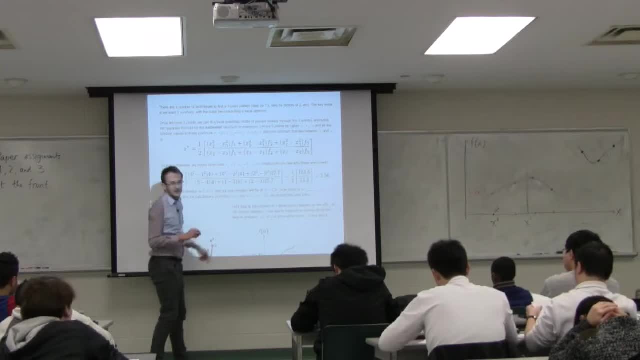 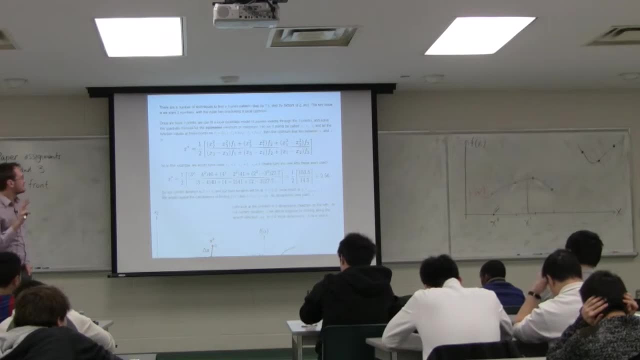 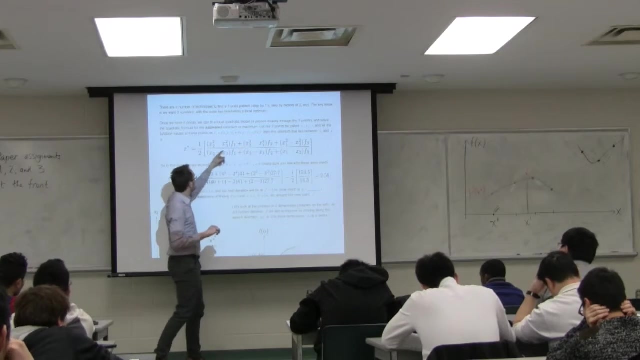 f1, f2, f3, evaluated at three levels of x, x1, x2, x3.. So take your three-point pattern, identify any x1, x2, x3 values, Evaluate the function at x1, x2, x3. 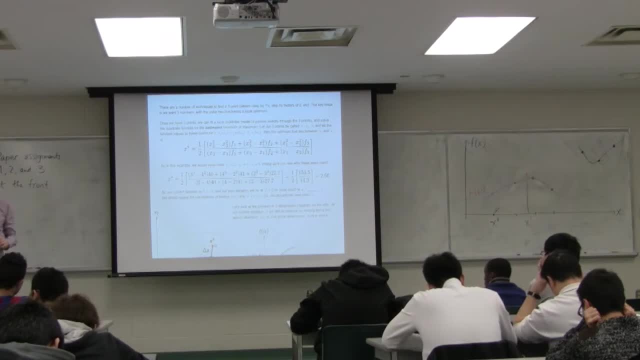 And this point here, x star is the optimum of that quadratic. So this is the solution to the quadratic equation for three values of x and three function values: f1, f2, f3.. So in this particular example, if I sub in: 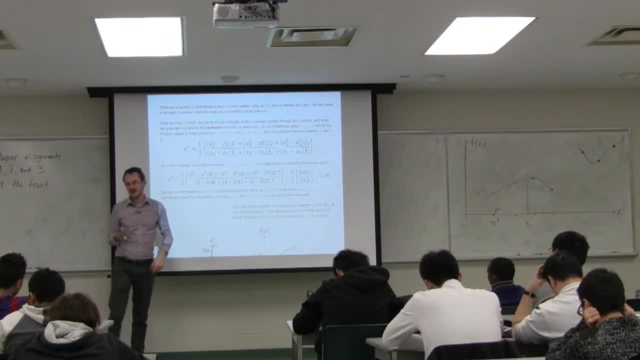 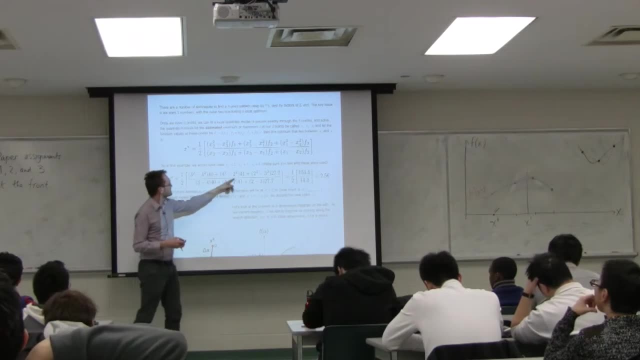 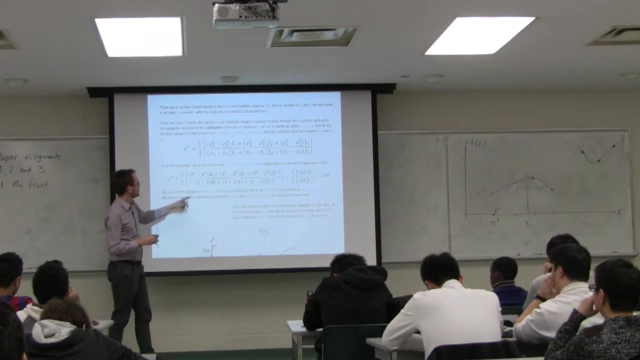 if I use x2, x3, x4.. x4 as the location for my three-point pattern, x1 is equal to 2.. I sub in that over there. f1 is the function value when x1 is evaluated. So that's why you see 40,, 41, and 27.7 over there. 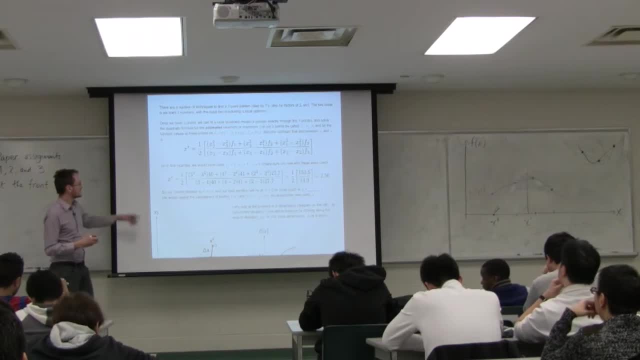 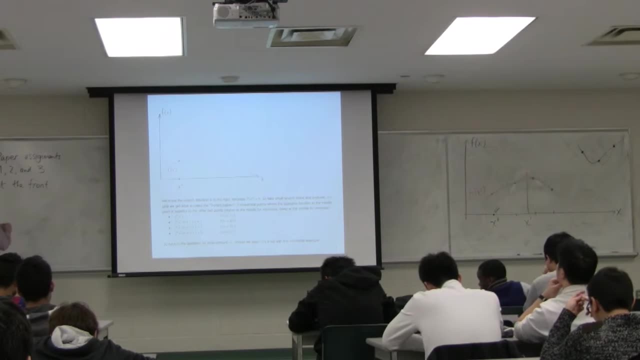 We can evaluate that And we get in this particular case that x star is 2.56.. So let's just go back to that data here at the bottom of the prior page. Make a note here that x star is 2.56.. 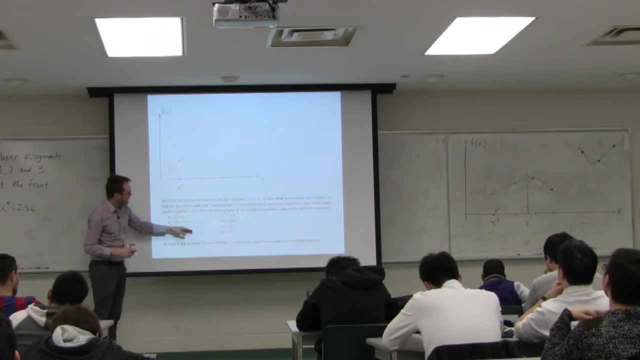 What we notice, then, is that our optimum- we're fitting our quadratic using these last three bullet points. Our optimum is at 2.56, somewhere between 2 and 3, between 40 and 41. OK, so that makes sense. 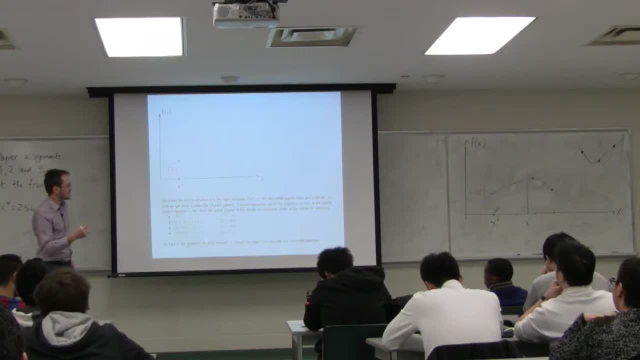 The quadratic starts at 40,, it peaks a little bit, passes down through 41, and then even lower still at 27.7.. So what was the result? It was 2.56.. What was my alpha then? 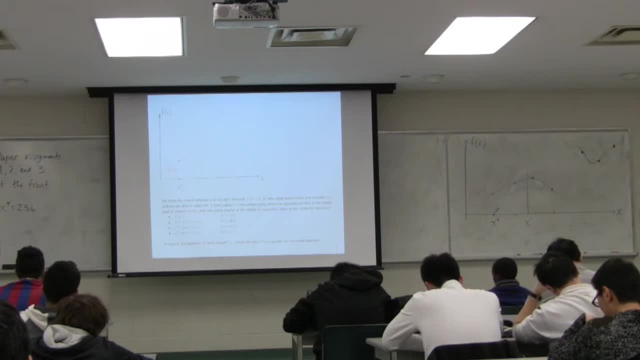 So my optimum x star was at 2.56.. What was alpha 1.56.? OK, So notice here that x0, my base case was 1.. If I take a step of alpha, that's, x is equal to 2.. 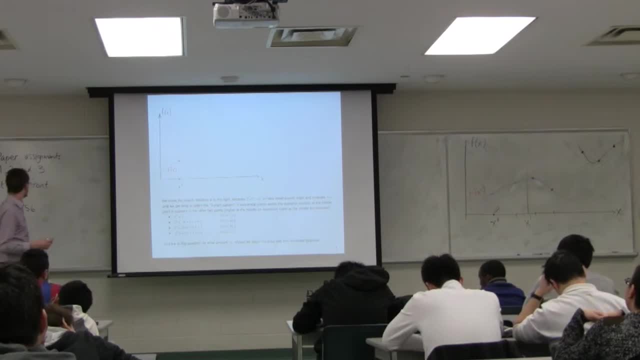 If I take a step of 2, alpha x is equal to 3, and so on. So, So If x star is 2.56, in this particular example, I took a step of alpha 1.56.. So, essentially, what we've done is: here's my slope function. 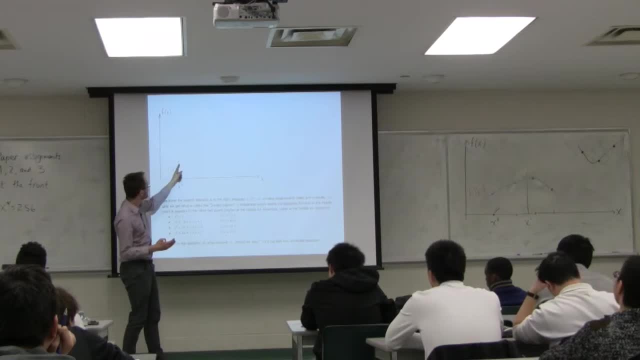 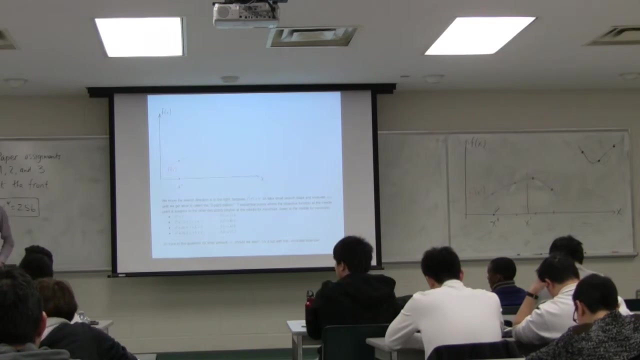 I've taken a step of 1.56 units from here- from x0, out in that direction. It happens to coincide with the point x star equals 2.56.. OK, and that point x star equal to 2.56 will become my starting. 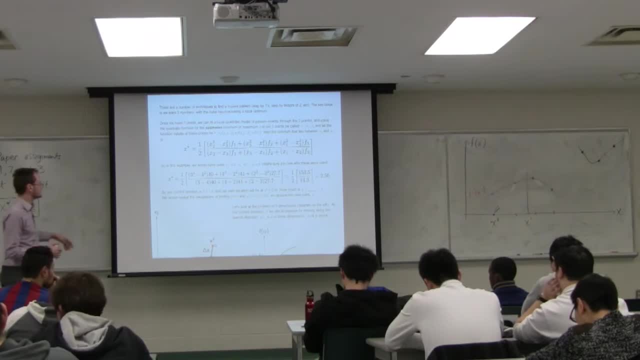 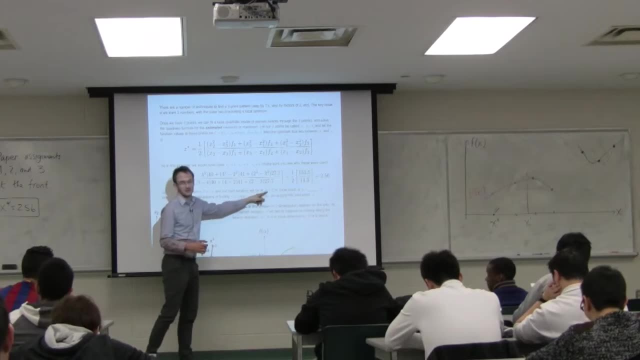 point For the next iteration. So here I've written that x star is 2.56, x0 is 1.. My next iteration will be at 2.56.. And at that point, 2.56, you're going. 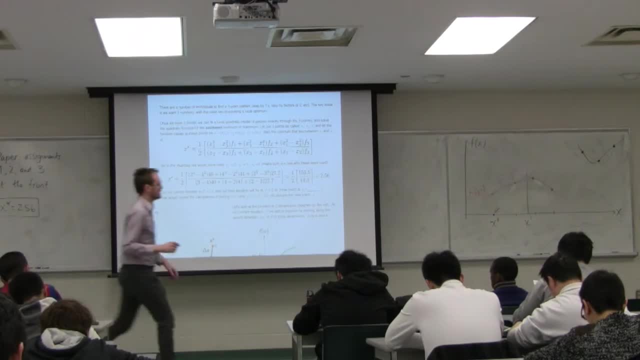 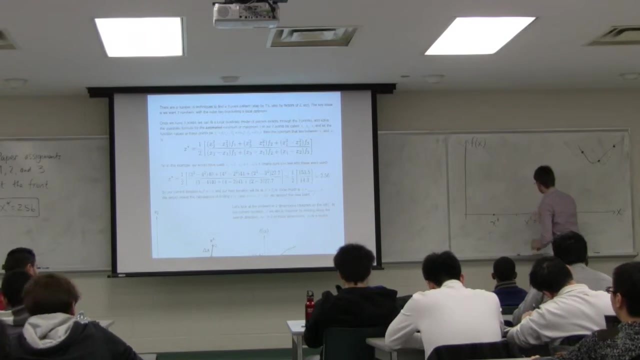 to find the function derivative. So let's perhaps just wipe this all out and illustrate how this will proceed for the next iteration. So x1 equals 2.56.. 2.56.. This process starts all over again. I'll explain it in a minute. 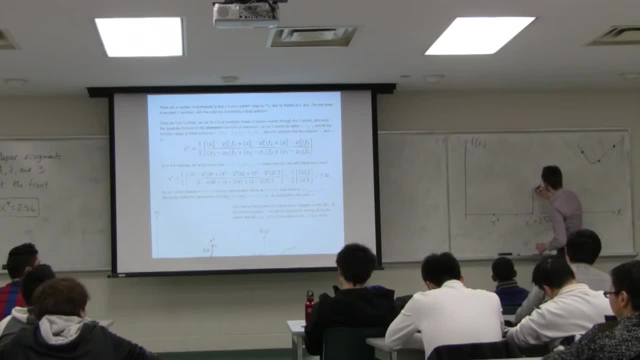 So x1 is 2.56.. I'm going to evaluate my function at that point, Calculate the first derivative f dash of x1. And then I'm going to start hunting for the optimum from this point on. OK, Mark wanted to know. so x? my first iteration was at 1, right. 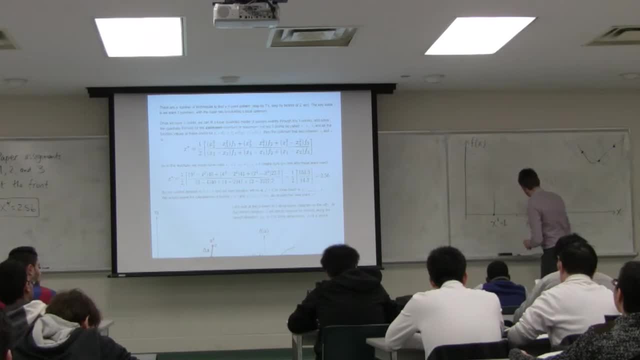 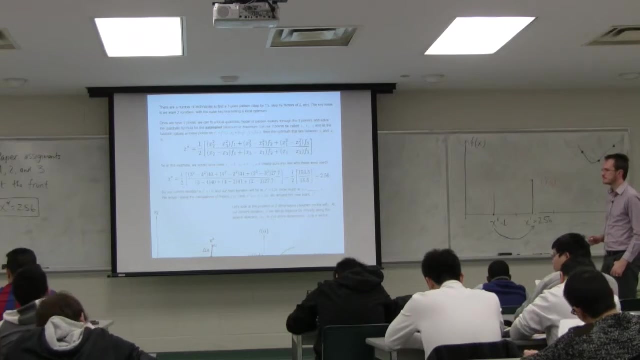 So x0 equals to 1.. So I stepped out a value from here to there. That's a step of 1.56.. If you go to the equation, on the first page you have x0 plus alpha And then the second one is x0 plus 2 alpha. 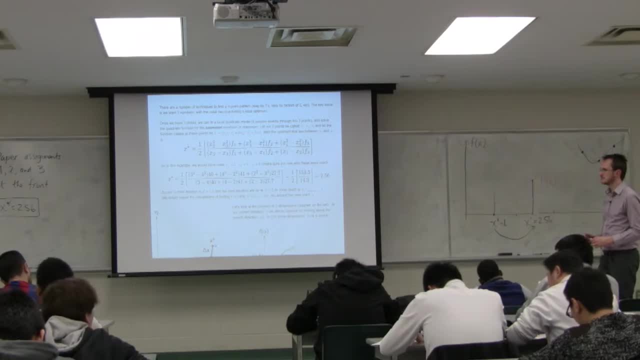 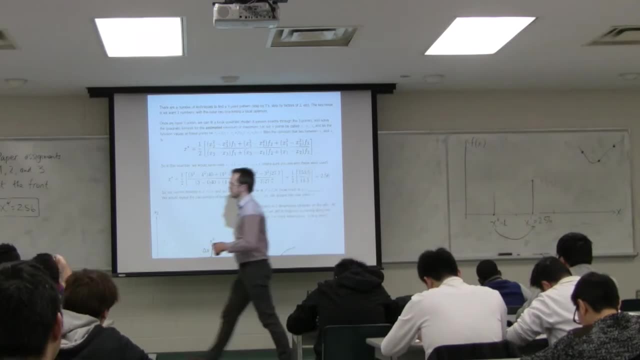 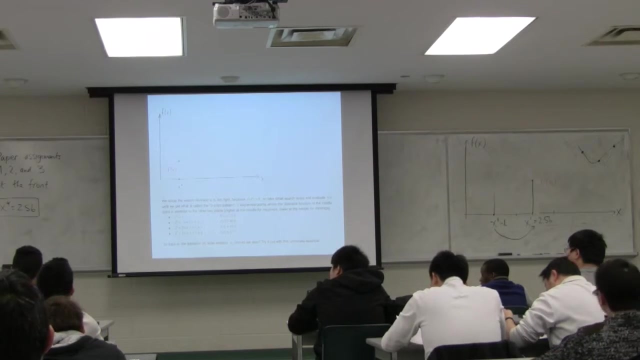 Yep, If alpha is 1.56, that doesn't really add up. Oh, OK, OK, I'm seeing the confusion now. OK, yeah, OK, I'm getting this. Yeah, I should probably not have said this. 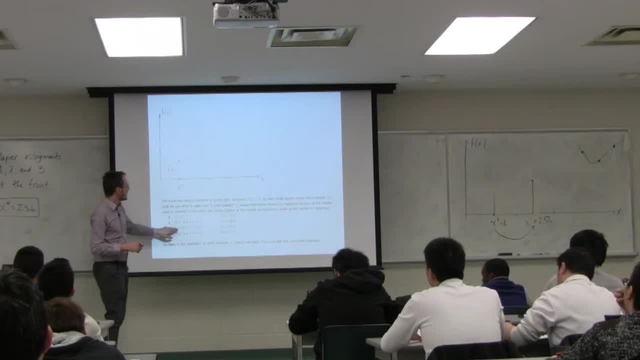 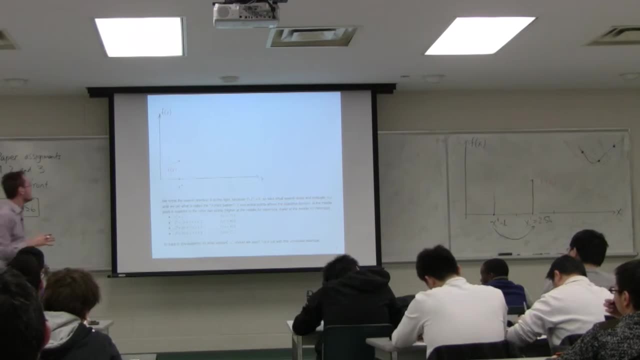 I should have probably this. OK, Why? Because I'm talking for the past five minutes and I'm seeing a lot of confused faces, So now that makes sense, OK. so let's see What I had intended to talk about here. 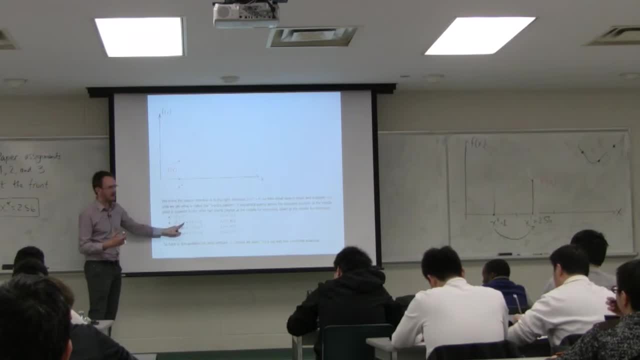 is that this is my starting point and that's a step away by an alpha amount. Here I'm stepping by two alpha units, Here I'm stepping by three alpha units. I'm taking steps of one at a time To find the optimum. I took a step of 1.56.. 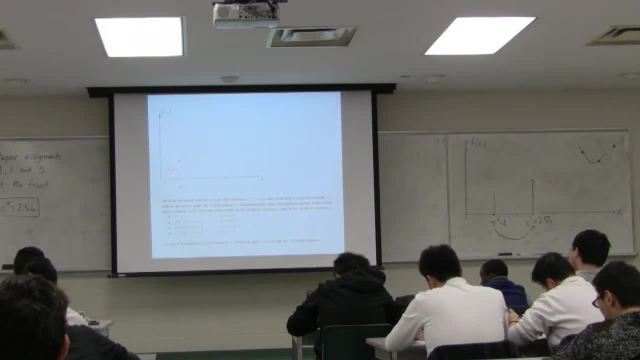 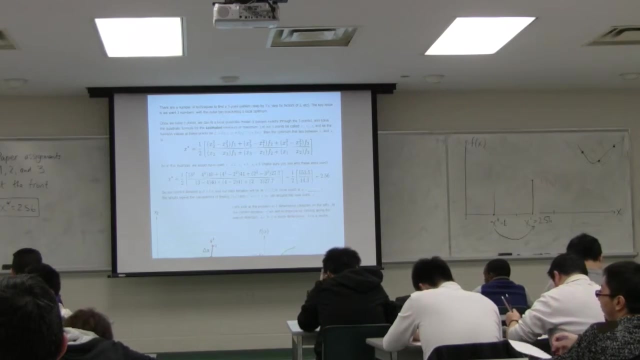 OK, that would be a better way of explaining what I've been trying to get across. OK, so what we're doing here is essentially building a local quadratic model for this unknown function And we're optimizing that quadratic model. The optimum for the quadratic model is at this location: x star. 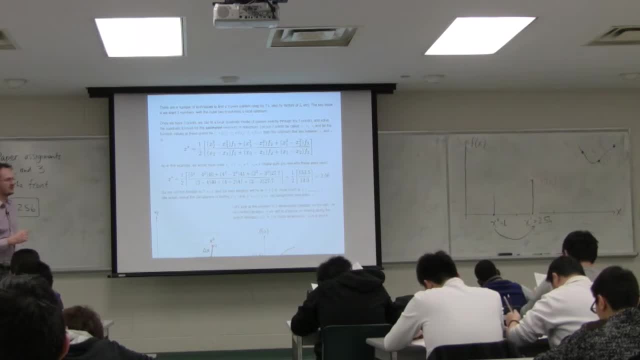 And our next iteration will proceed starting at that point. So apologies if that didn't make sense, But the idea is that we build a local model, OK, OK, Let's take a look at this perhaps in the multidimensional sense, So you're getting a second chance to try and understand. 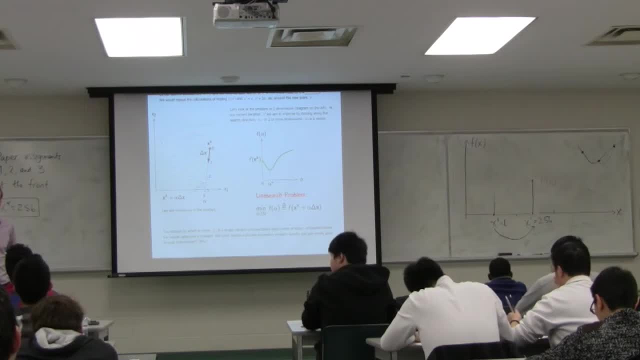 this concept in two dimensions. Before you start with x: if you start with 2.56, is your next alpha step also 1.56? Or do you just No? At the next iteration it's 1.56.. 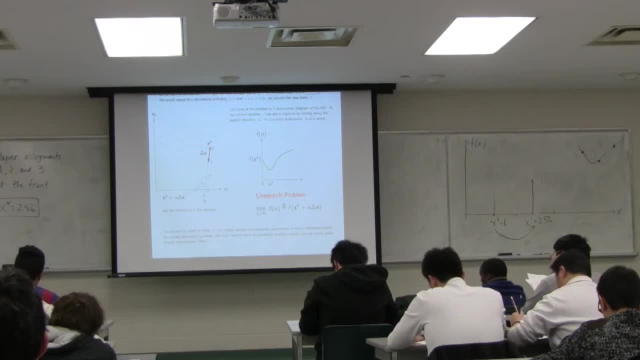 You can start searching by a different amount alpha, And we're going to actually see that here in the two-dimensional example: The first time we search we'll get a different alpha to the second time that we search. OK, So it might be a little easier in two dimensions. 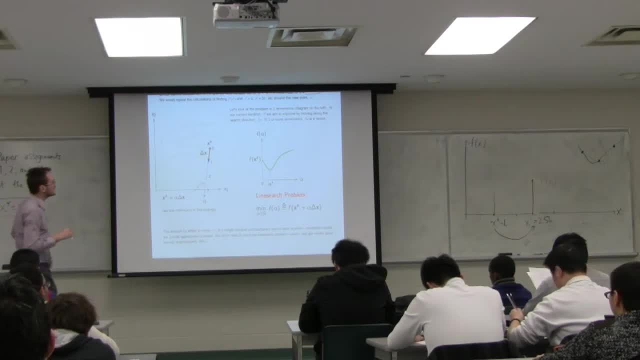 especially because you're seeing it another time. So in two dimensions we're starting at this particular location over here And the search direction is given by the slope right, In the same way that here The search direction is given by the slope f. dash of x. 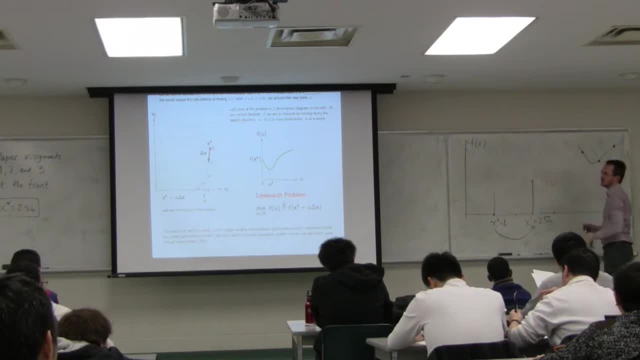 The fact that f dash of x is in this direction tells us to keep going up the mountain. OK, In two dimensions. we just don't call our search direction f dash of x. We replace that with the partial derivatives of f with respect to x. 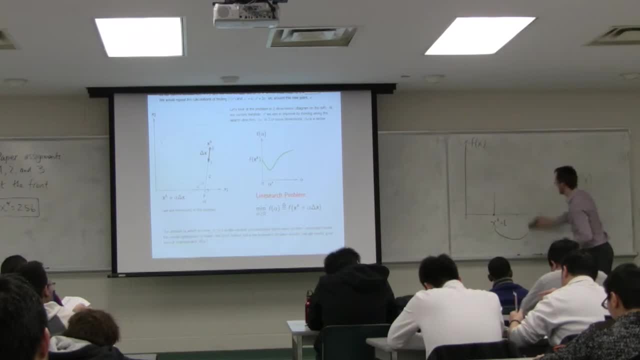 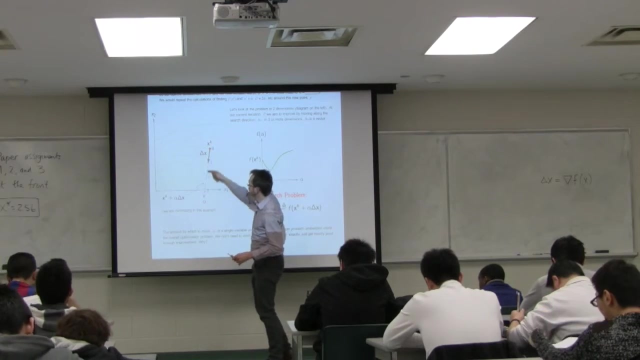 But it's still the same meaning. It's the tangent or the slope at that point. OK, So that's my search direction, delta x, And we're asking: how far along this direction do we go? We saw this in the prior class, that if I'm at this point, 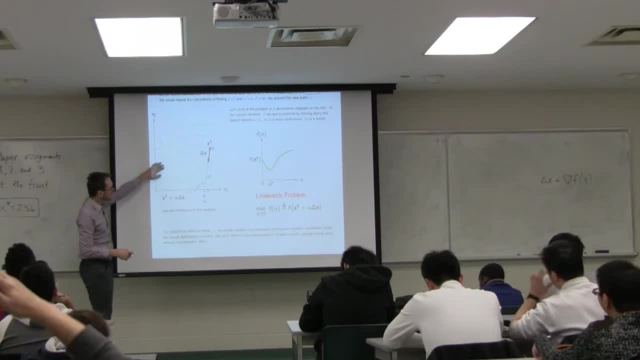 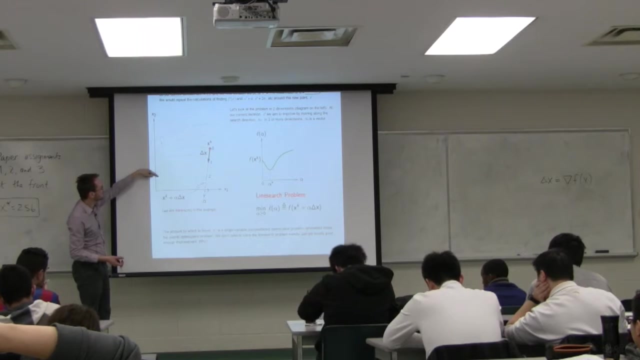 and these contour lines in green point to a minimum right. So the objective In this particular function- excuse the spelling error- is we're trying to minimize this example. We're trying to find the valley at that local point over there. I'm currently at this iteration at the red dot. 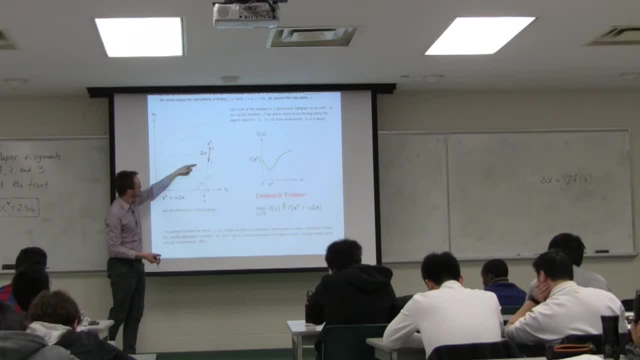 And the gradient tells me to head down this direction. So if we looked at this function and moved along that dash blue line, this is actually what we would see here in the graph on the right. We're at that location of f And if we're 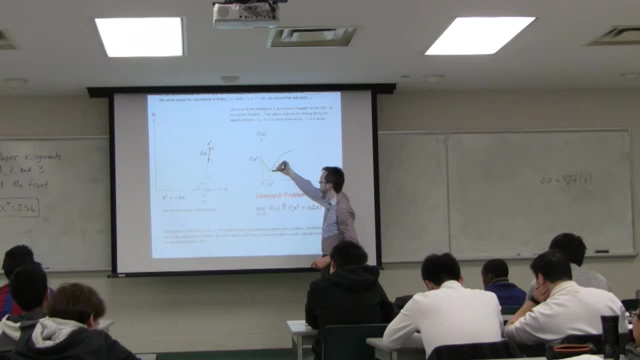 moving along that dash blue line, our function starts to decrease, But if we keep going more, we start to actually climb up the mountain again out of the valley. Our goal, then, is to find this amount alpha star. How much of a step do we take? 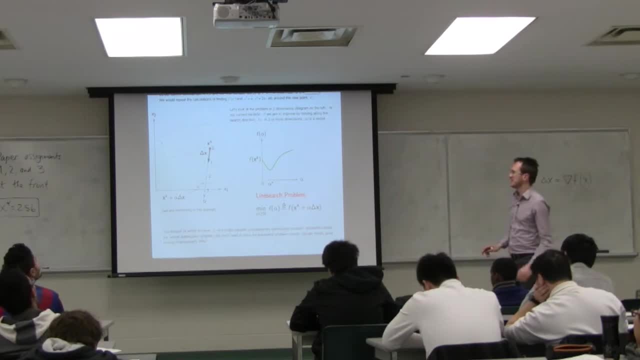 And that was what I tried to describe in the prior page- in a single dimension. Here we're doing this in two dimensions. We're changing a little bit of x1. And we're changing a little bit of x2. At the same time, 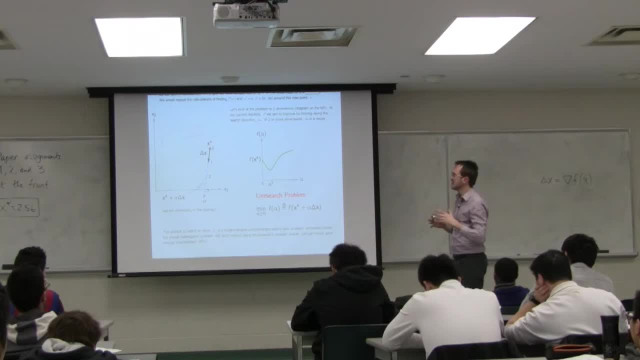 In the prior example you only had one x to deal with In two dimensions. you change both x1 and x2 by some amount in this constant ratio along that vector. So if you step x1 by a certain amount, you have to step x2 by a certain amount. 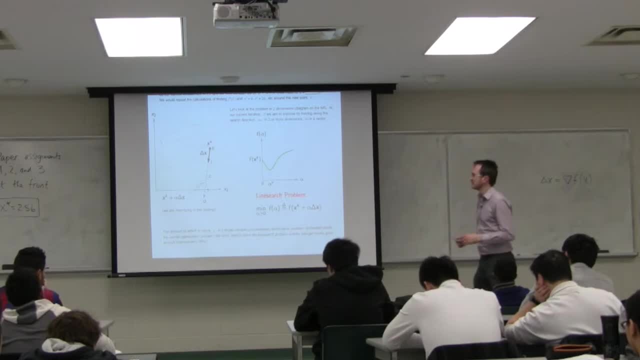 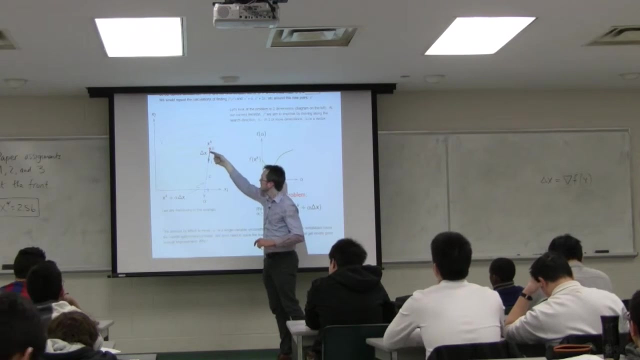 to remain on that dash blue line And that's your search direction, or your direction of steepest descent, Which is this slope at the point? It's exactly right, It's your slope at that particular location. So it's telling you that if you want to head downhill. 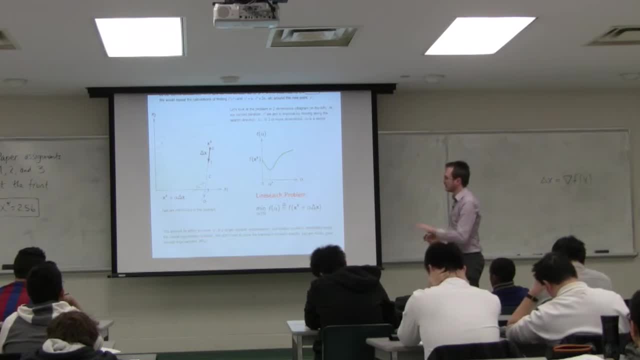 go in that direction And then you'll go downhill, But what you see is that if you go any further, you start to go uphill. So our goal, then, is: we've changed our goal from trying to find this minimum to solving a little bit of a different problem. 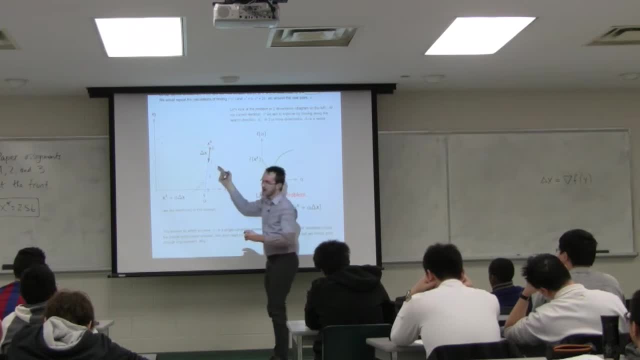 We want to find where that lowest point is. When we find that lowest point, let's call it alpha star, and it's going to be somewhere around over here. We're going to then stop, recalculate our slope and then start to head in this direction. 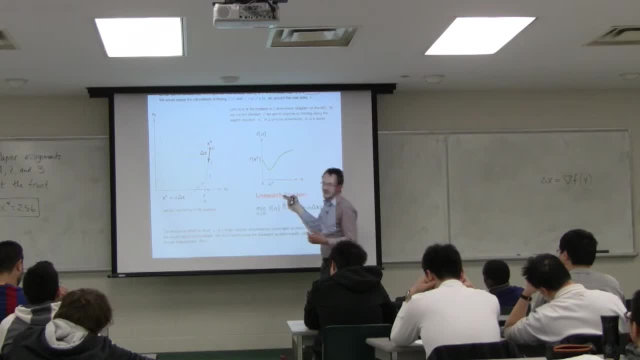 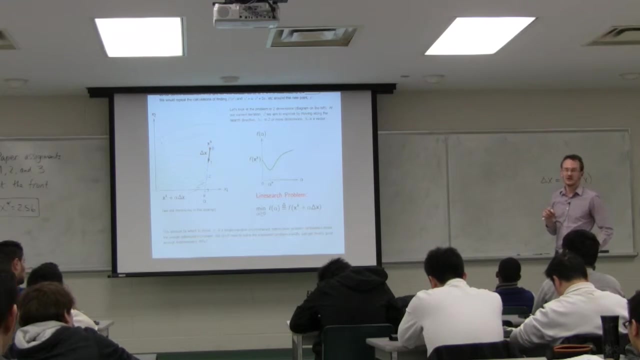 by a certain amount. So what the line search does is: it prevents you from going too far and deviating from your goal of seeking out the optimum. The key point I want to emphasize is that line searches don't have to be solved exactly. You can solve it, even just approximately. 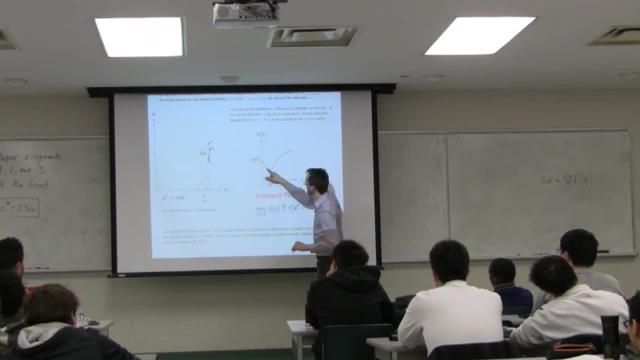 but you don't have to solve it exactly Right. It's no point in trying to spend a lot of computational effort to find exactly where that minimum is, because you're solving this problem of finding the minimum along this path, Even if you're approximately correct. 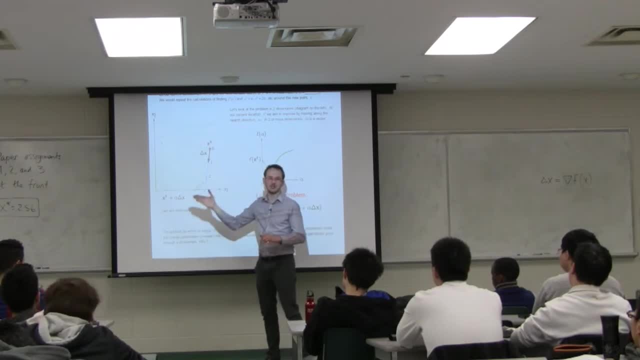 you're OK, because you're going to reiterate, recalculate the slope and readjust your search direction. So it's kind of like finding directions, say, from Toronto to Montreal. There's any number of paths you can take, but you can go from, say, Toronto to one other town. 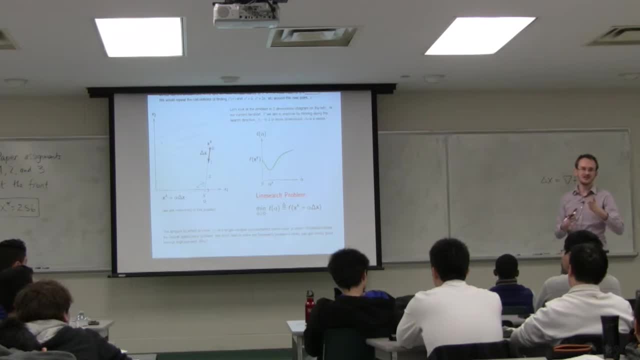 along the way- Belleville, for example- and then re-optimize at that location. Take another step, re-optimize, keep going in that direction. You'll eventually get to your goal. There's no sense in trying to find the exact path. that's. 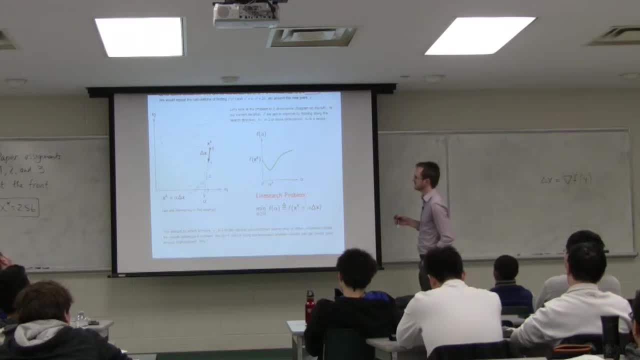 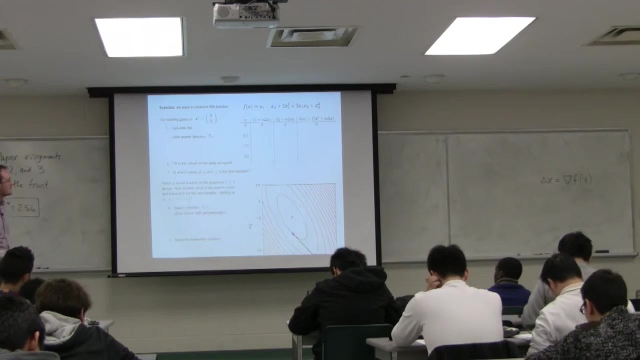 optimum because of these repeated iterations. So let's see how we do that. I'm going to give you an exercise here to try. I'm going to give you an exercise to try it out with. Here's a function: f of x, up there on the top of the page. 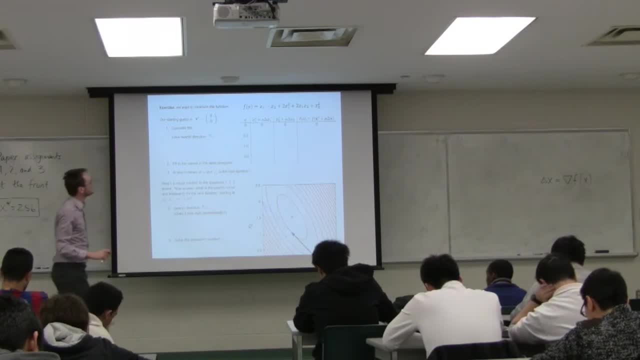 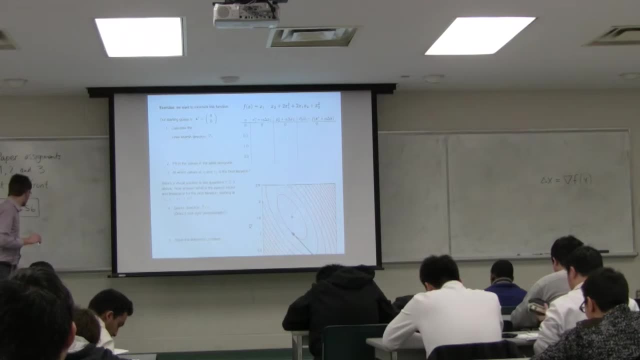 And we're going to start at the simplest point, the 0, 0 point. So the first step I'd like you to do is we're trying to minimize this function f of x. So minimize f of x, find then the search. 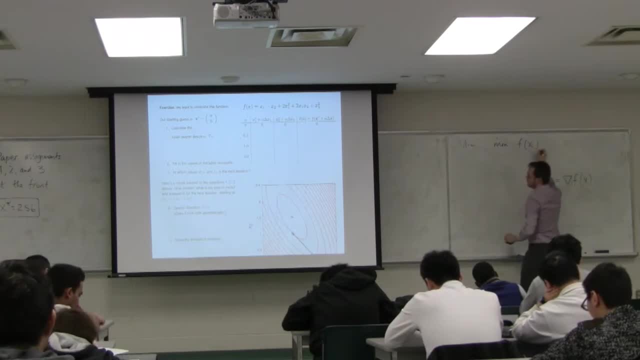 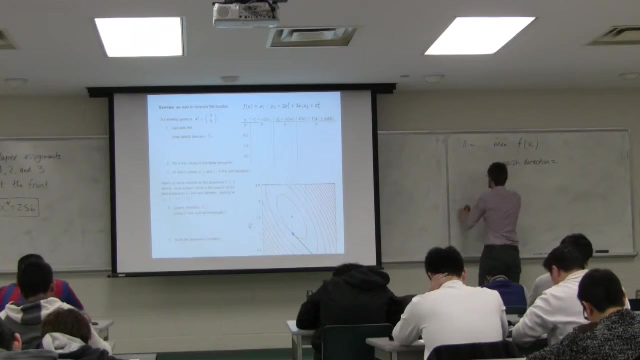 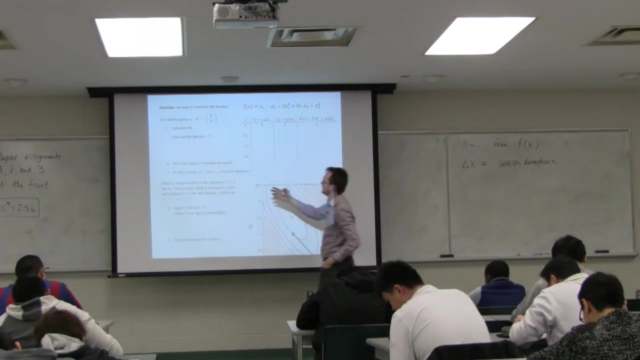 direction that we're going to move from, starting at 0, 0.. Here's a geometric picture further down the page, but you could do this analytically, So I'll give you some time to do that. Yeah, please, I just realized that triangle's. 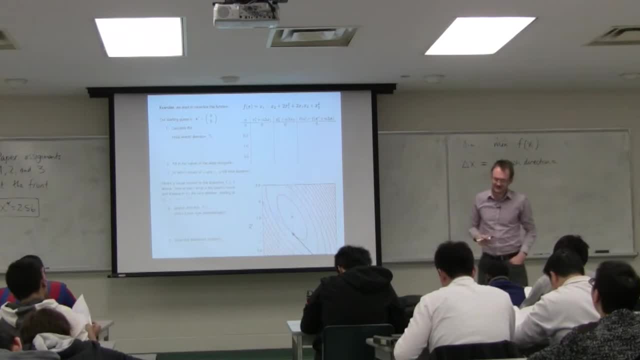 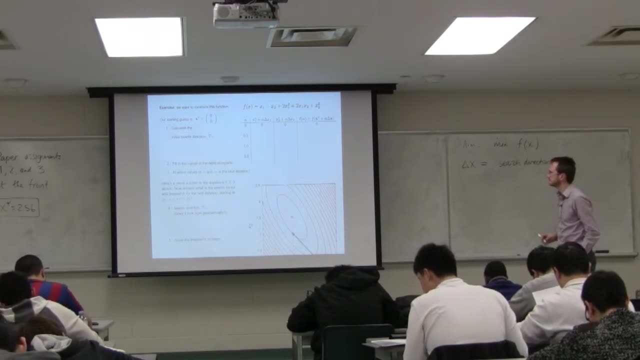 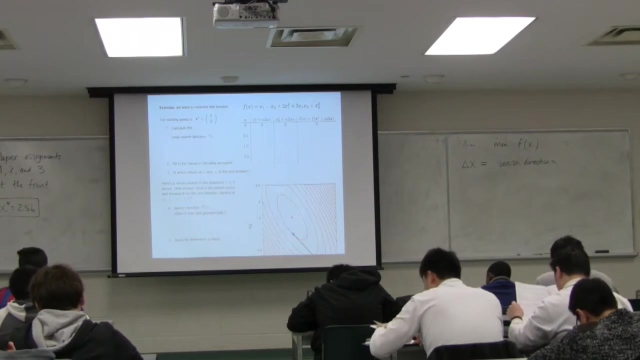 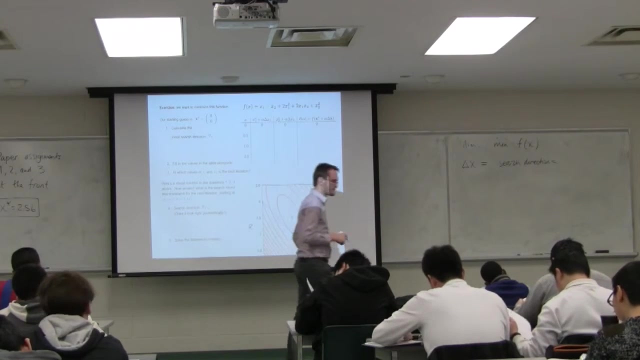 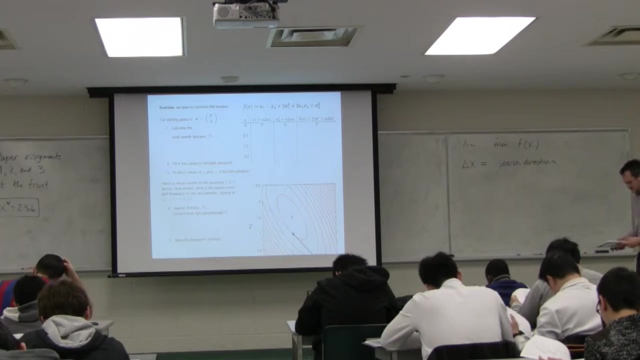 the wrong way around. It's the regular direction. OK, the answer to question 1 is right at the top of the handouts on the prior page, page 1, where we said what our search directions are. OK, there we go. 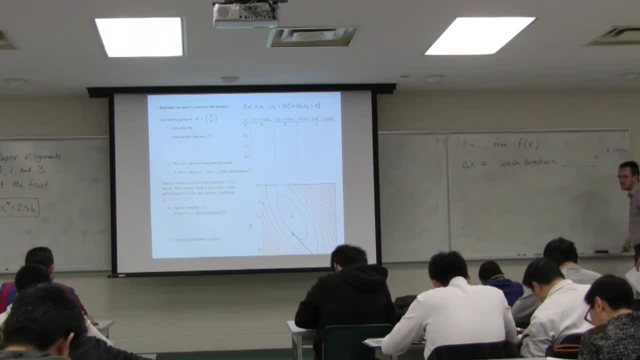 so search directions are a vector. you must get a vector here in this answer. so okay, so your search direction recall is equal to the negative of of the gradient we're trying to minimize. so you must have that negative over there. the upside down triangle f of x refers to: 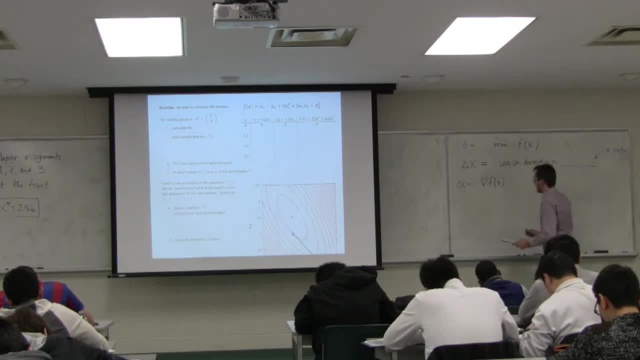 the partial derivatives of f. so let's just actually write that out here: partial derivatives of f is a vector, so that's the df by dx1 and the partial with respect to x2 is what that's saying mathematically. so the first partial derivative, then you can calculate that. 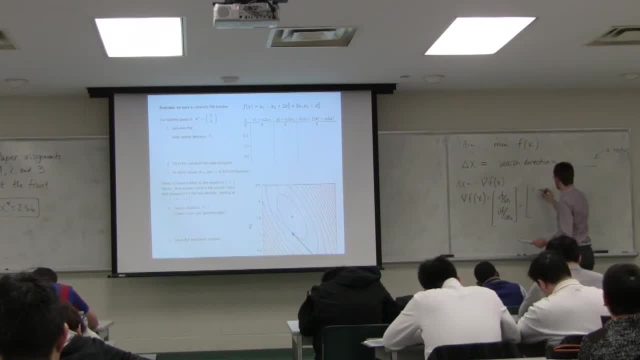 is equal to 1 plus 4x1 plus 2x2, and the second partial with respect to x2 is minus 1 plus 2x1 plus 2x2. so you should have at least calculated those, and then what we're saying is that 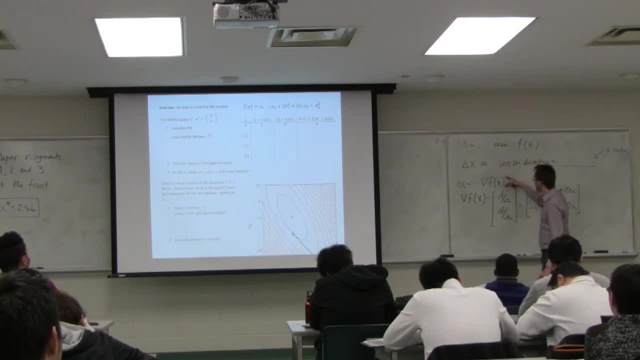 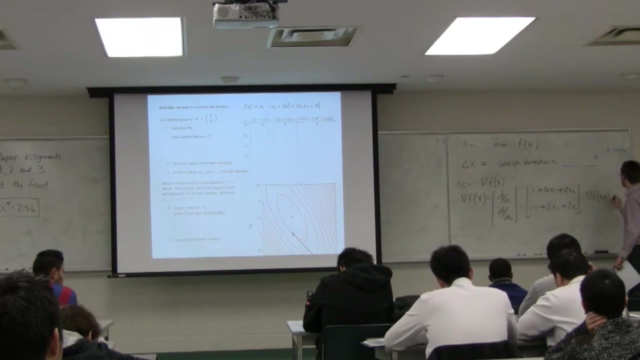 that search direction is: evaluate that partial derivative function. at our current location we're at 0,0, so let's just sub in then that delta f of 0,0 is equal to 1 and minus 1. okay, so therefore our search direction: delta x is equal to the negative. 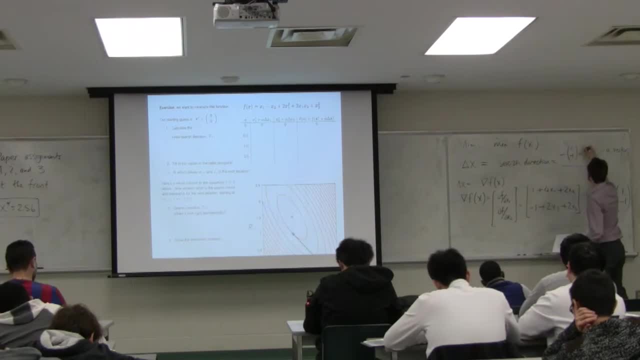 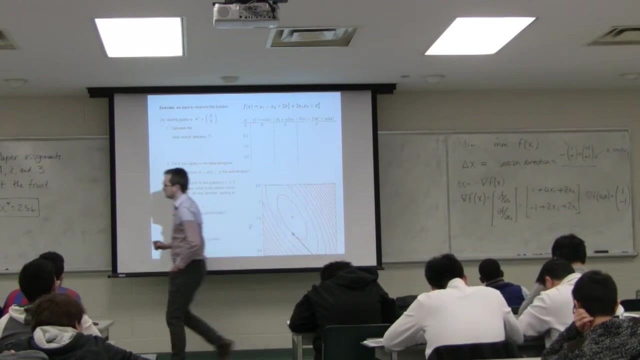 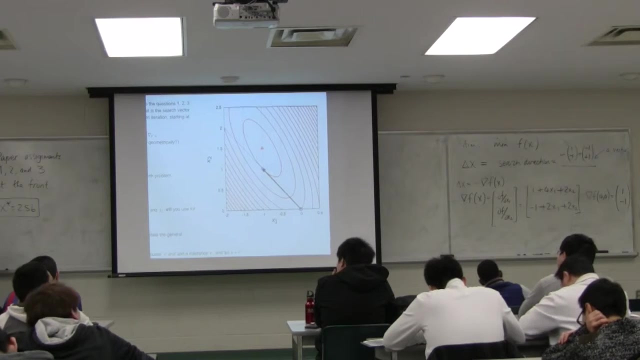 of x2, of that, 1 and minus 1 is equal to minus 1 plus 1. okay, now, before we move on from that it we shouldn't just calculate these things without trying to make sure that they're right. Let's see what we're doing here: geometrically right. 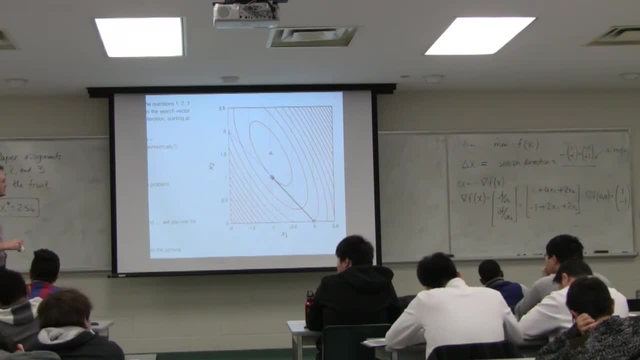 So again, I'll emphasize: the computer doesn't do this, but we can do this to learn what's going on. In red are the contour lines of the function we're trying to minimize, And the minimum is drawn here for us in the triangle point. 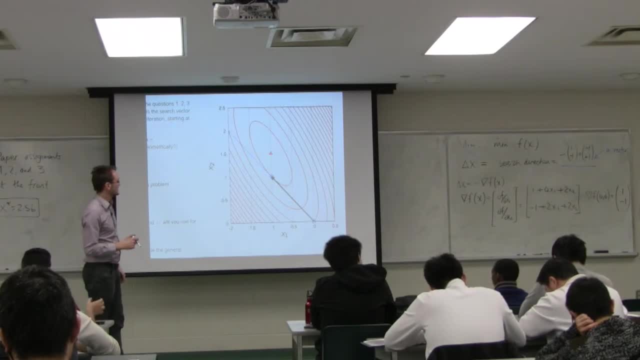 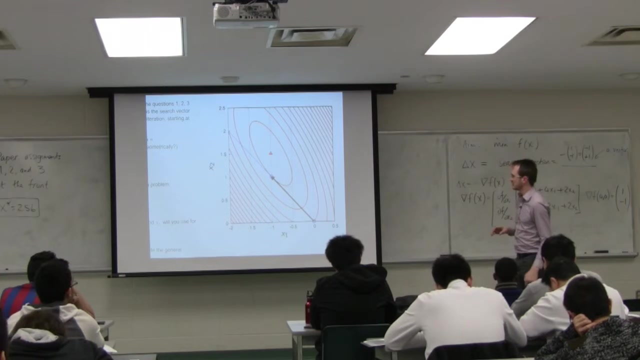 Our current guess for where we're starting is 0, 0.. So x1, 0, x2, 0. So that blue circle over there on the bottom of the graph Now search directions, we know, go perpendicular to the contour lines. 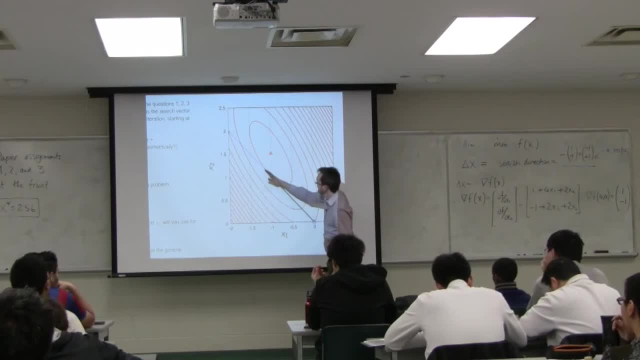 And we actually see that here. We're heading perpendicular to the contour lines, But notice here that the search direction here in blue just simply tells us to go along that direction, but not how far. So we haven't even answered that question yet: how far. 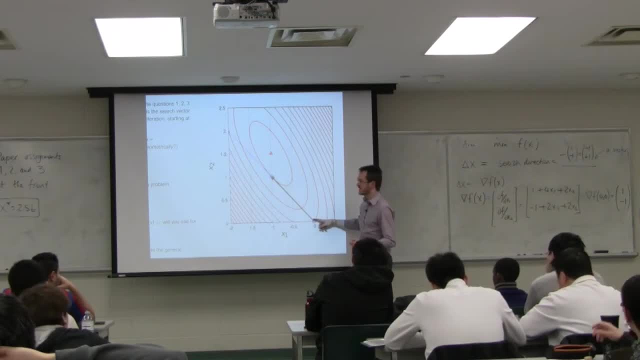 We're going to look at that next. I just want to verify First that our search direction actually is reasonable. It says: step negatively in x1 and positively in x2.. So at the very least the signs have to agree, right. 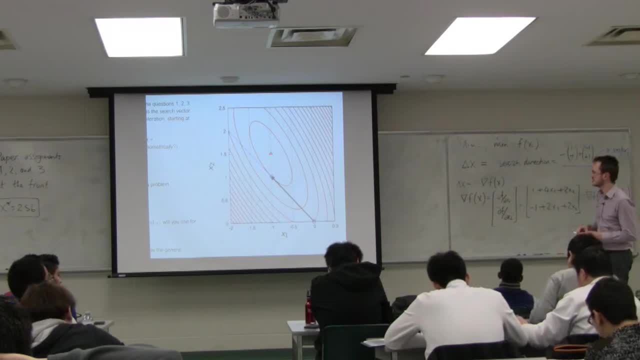 If the signs don't agree, you know that right away that you've made a calculation error. So it says: go decrease x1 from where you currently are. So x1 must go negative. We observe that And make x2 go up. 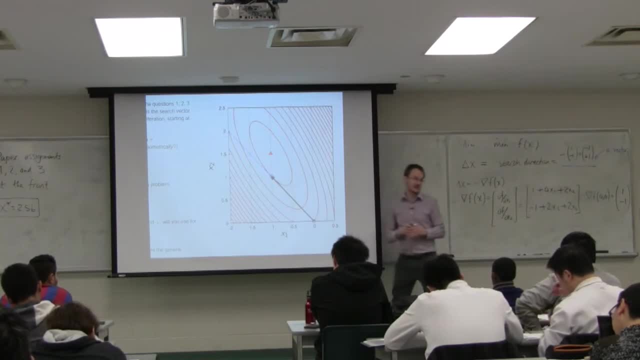 We're at 0. And we see that x2 heads up. So the signs agree. Let's take a look at the magnitudes. It says if you take a negative 1 step in x1, you must also take a plus 1 step in x2.. 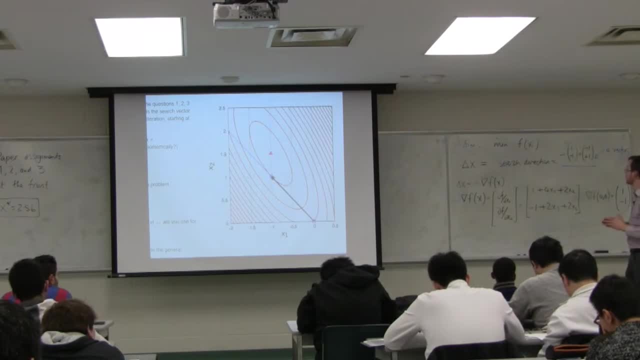 You have to obey that relationship in order to go along that search direction. So we see there that for every minus 1 step we take in x1, so I'm going from 0 to minus 1, for example, I must take a plus 1 step in x2.. 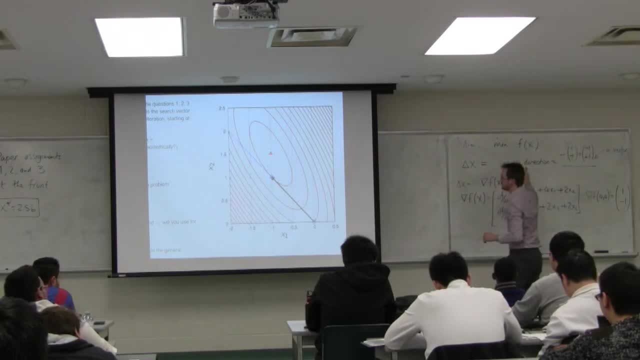 If I decided to take a step of 2 units in that direction, ie from 0 to minus 2, I must make a plus 2 change in x2.. So I go from 0 to 1, okay, So any point along this blue line satisfies that relationship. 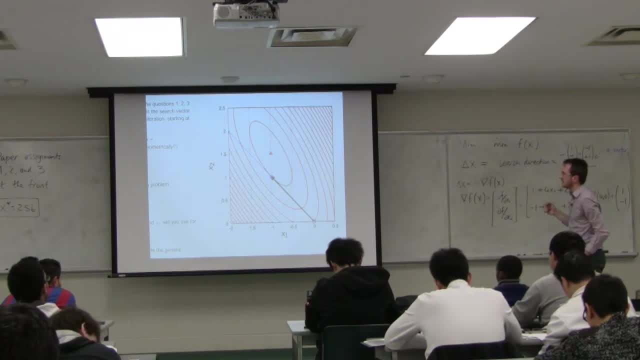 of staying along the minus 1, plus 1 vector. So that is intuitive to us. The next question is: how far? If we look at these contours- starting out here at 0, 0, we can see that we decrease, decrease, decrease, decrease. 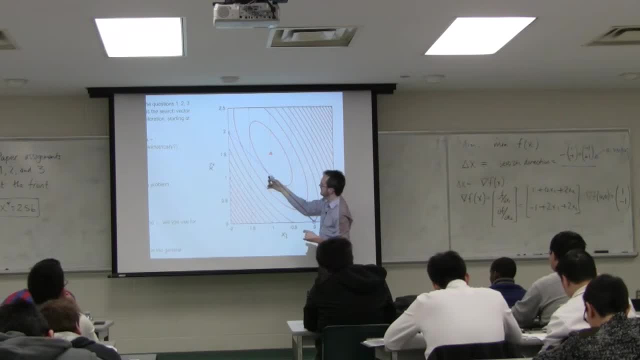 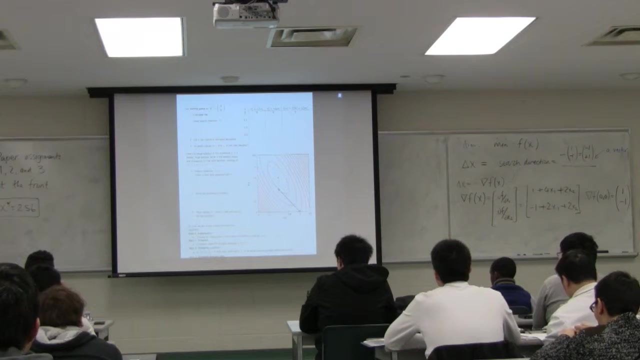 And in fact, after we go beyond that blue circle over there, we start to go back up the contours again. So there's a minimum along this vector. We just don't know where, And that's where we use this table And a computer. solving this would do exactly the same step. 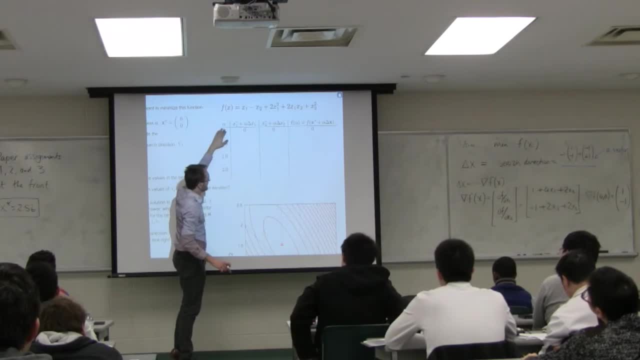 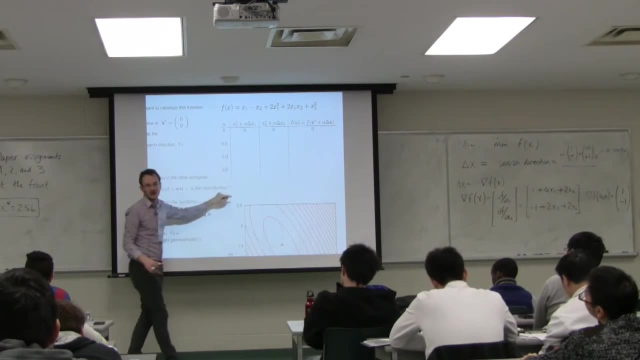 The computer would say: right, I'm here at 0. At that point let me go and take a step of half an alpha, of 1 alpha, of 2 alpha, and evaluate the function along that line. So those function evaluations then show up here in the last column. 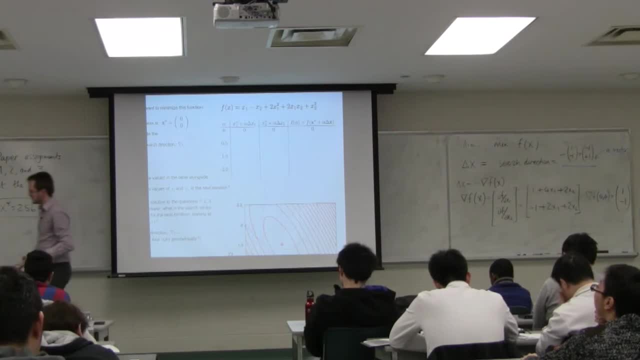 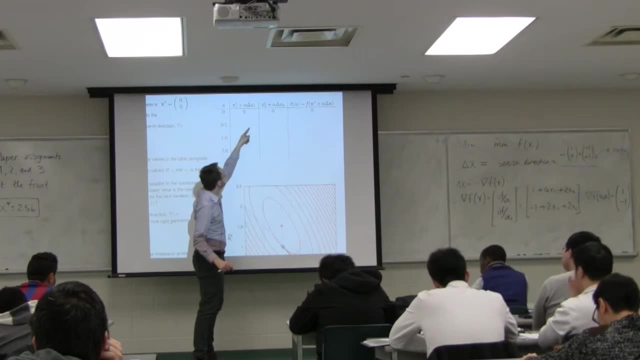 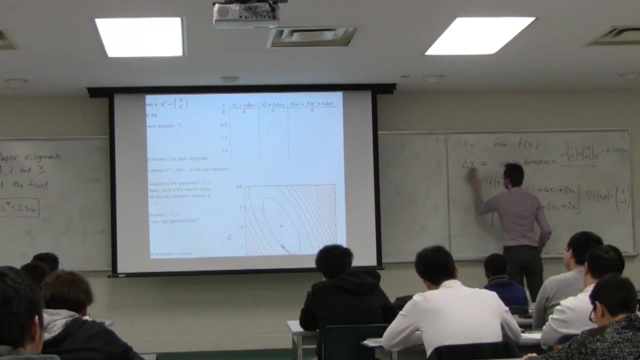 Now, when we take a step of half an alpha, what that says is to increment x1 by 0.5 times the search direction And x2 plus 0.5 times the search direction. So let's sub in that table there. 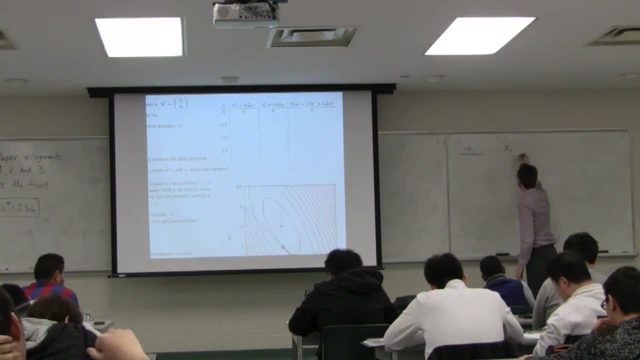 So, alpha, we're going to move x1.. We're at the 0th iteration. at my initial guess I'm going to take some step. alpha times the search direction For x1.. So let me maybe just record here: Delta x1,, delta x2.. 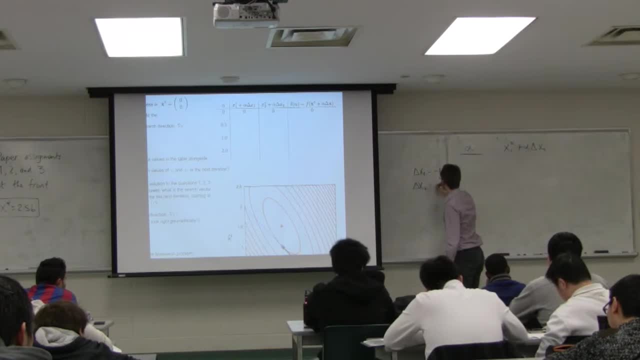 These are the search. directions are minus 1 and plus 1.. So I'm going to move some amount in x1. And I'm going to move some amount in x2.. So x2 at my initial condition, 0, plus alpha times delta x2.. 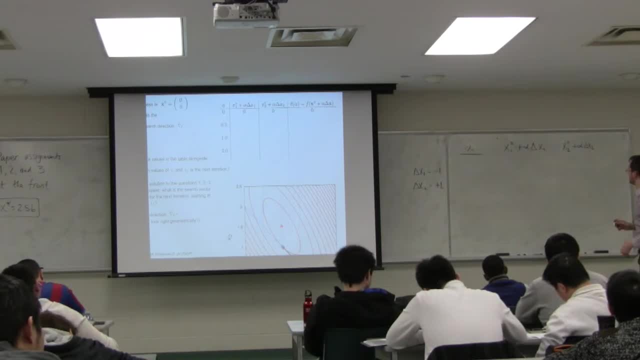 So subscripts refer to your variables, Superscripts refer to your iteration numbers And then at the last column I'm going to evaluate that function at that value of x1 and x2 in the prior columns. So when we're taking 0 step, our current x1 value is 0. 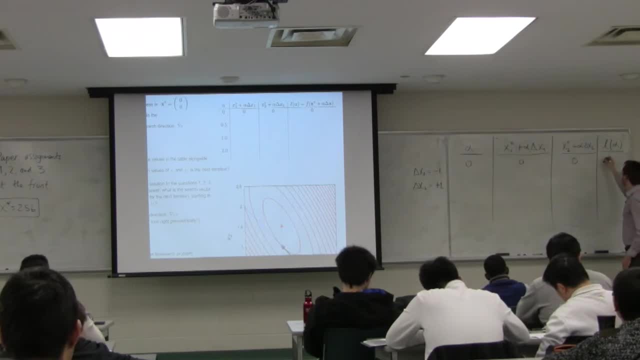 Our current x2 value is 0.. Evaluate f at 0, 0.. We get 0.. So that one's trivial. But if we decide to step by half an alpha, what's this entry over here in the second row, second column? 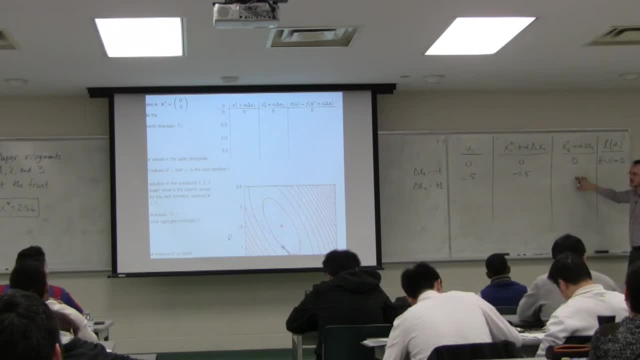 Minus 0.5.. The entry in the next column over Plus 0.5.. OK, And you can evaluate the function there as minus 0.75.. So we're decreasing. That's good right. So we're at that point. 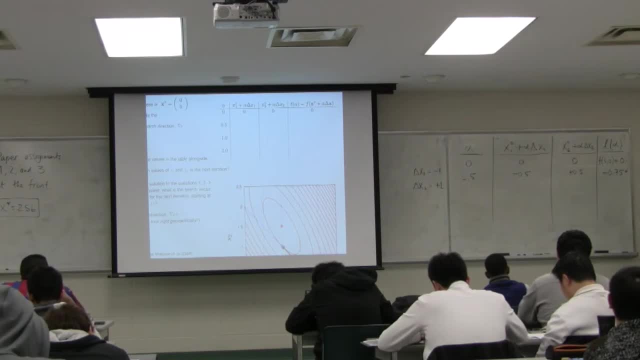 We're dropping. OK, Let's take another step of alpha. Let's take a step then of 1 alpha. So it says: take a full-size step. So that is minus 1 plus 1.. And f of minus 1 plus 1 is equal to minus 1.. 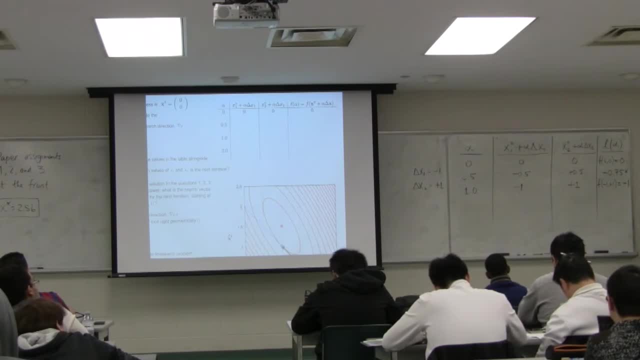 So we're going to get 0. And we're going to get 0.. OK, So that's again. that's OK. We're dropping even further. still Not as much as we did, but we're dropping OK. 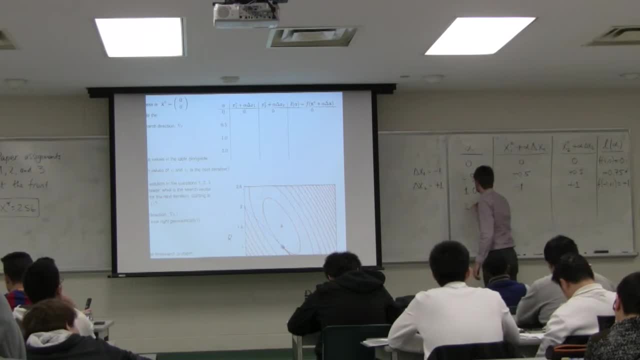 So we keep going. Let's take a step then, of 2 units, 2 alpha units, So that's at minus 2 and plus 2.. And then, when we evaluate f, at minus 2 plus 2, we get an answer of 0.. 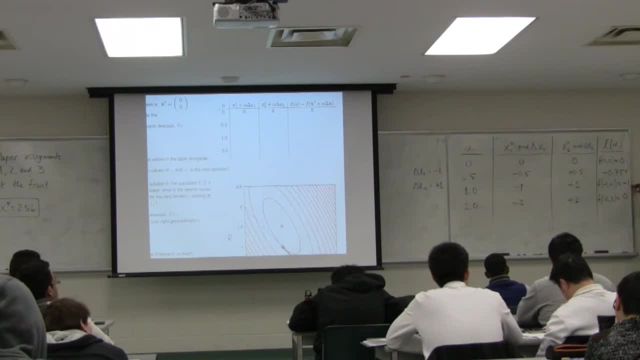 So we've gone down, We've gone down And now we've gone up again. So which three points would you use to try and fit the quadratic? We've got four points here on the board. Which of the three do we pick? 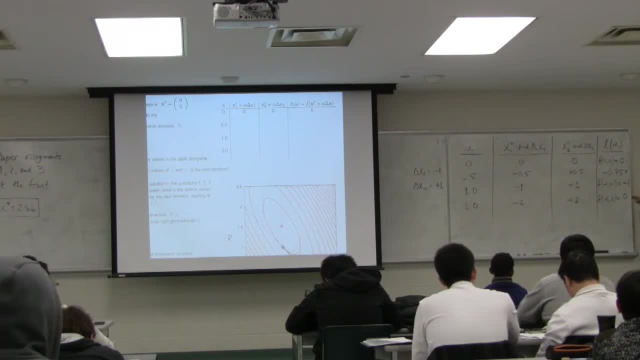 The last three. OK. So we pick the last three. Go fit the three-point problem. Just tedious mathematics, but it's doable, OK. And you will actually find it's coincidental in this particular example that the three-point optimum is at this entry over here. so at alpha equals 1.. 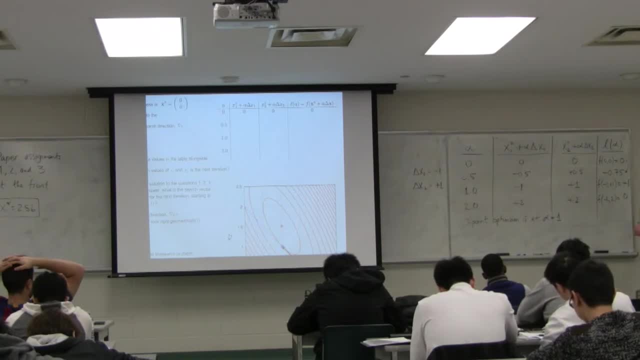 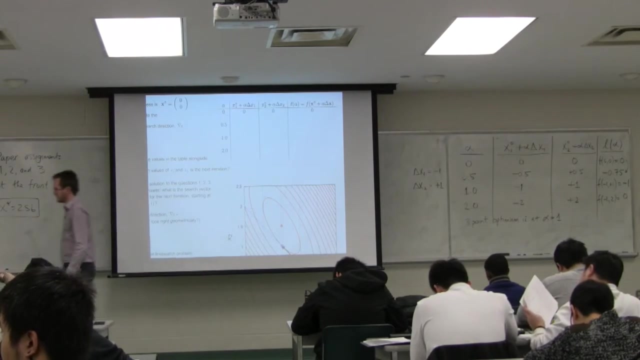 It's just coincidence, in this time It won't necessarily be one of the three points that it picks, but in this case it is OK. So my next iteration then starts at that location. So geometrically I've stepped from 0.. 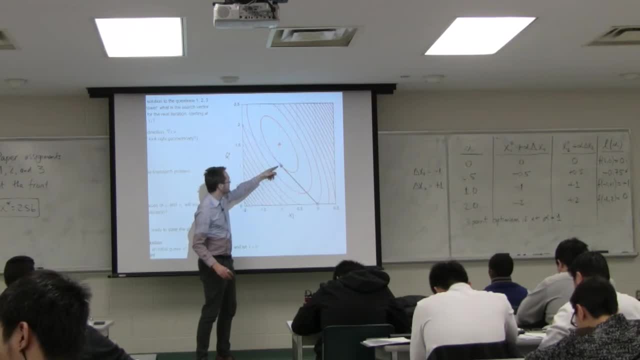 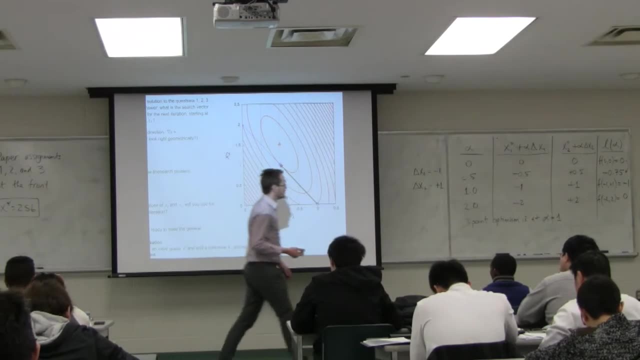 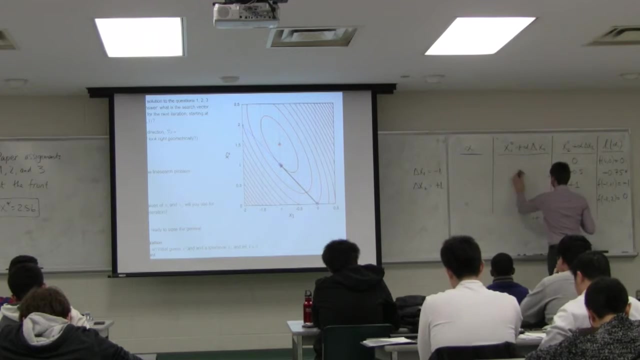 I've taken a full step of alpha 1.. That's where my optimum is And I'm going to relocate myself at that point So you can wipe this table clean And we're going to restart again. So I'm going to take the last one. 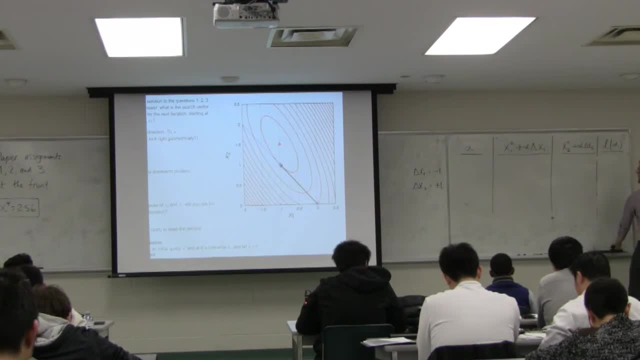 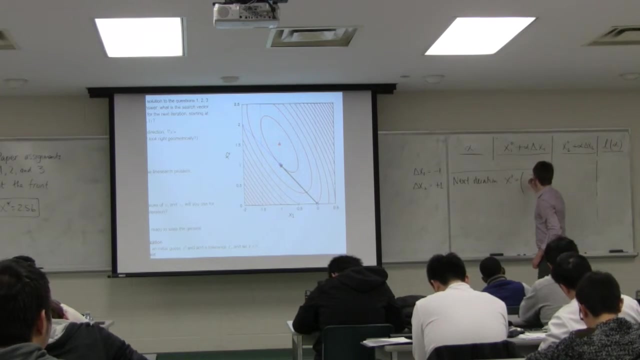 How did you guys get the last? It's just the function evaluations at these two values of x. So my next iteration, we can say the following, Let's just write it over here: My next iteration is x1. And x1 is equal to this location minus 1, plus 1.. 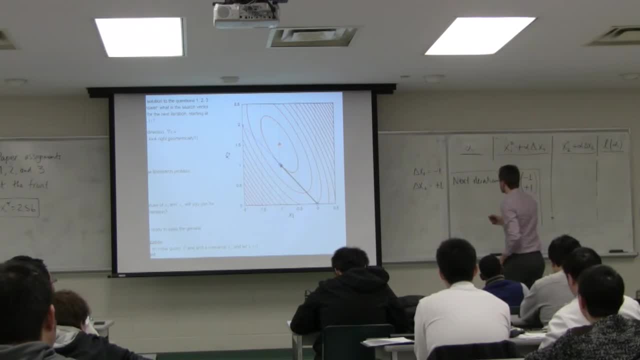 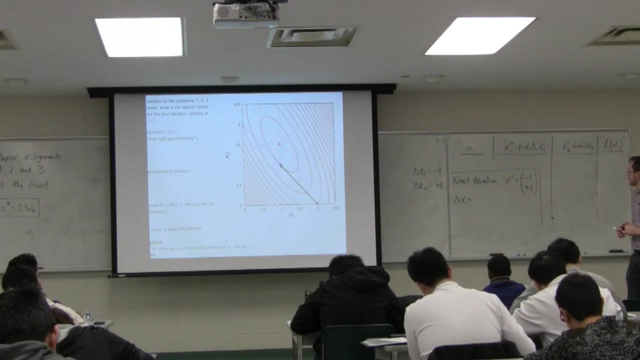 So start the process again. What is my search direction? I'll give you a minute or two to calculate that The process is: find search direction, find the line, search optimum. So this handling aspect takes a little bit long. I'm gonna take a little bit longer to collectively. 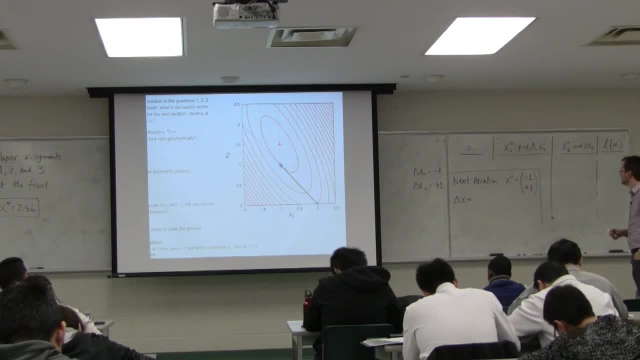 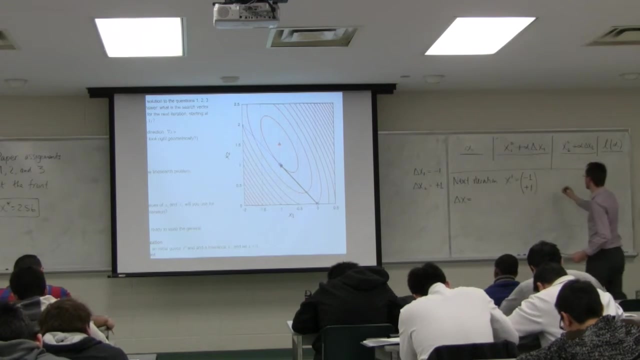 identify, and the methods I'll take might be a little bit complicated, But I always want to make sure I use a little bit of space, So Iそんな don't take much space And that okay. So let me juggle this together. 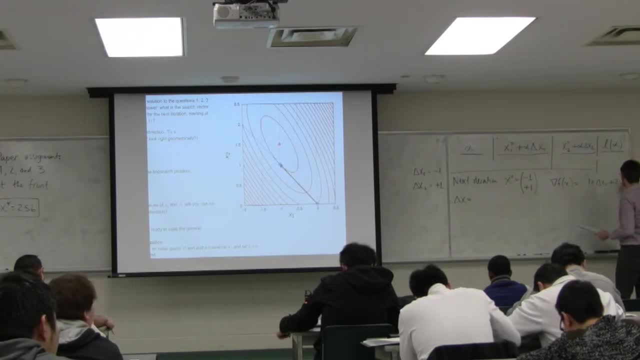 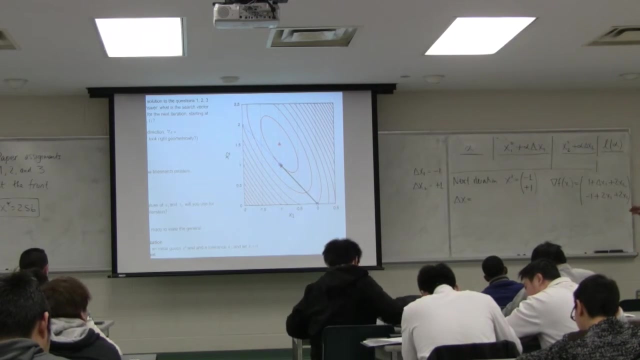 And I'm just steering. That's what I'll be doing, OK. Okay, when you're done calculating that, cross-check it with the person next to you to make sure you've got agreement. If you've already done that, you're welcome to move on. 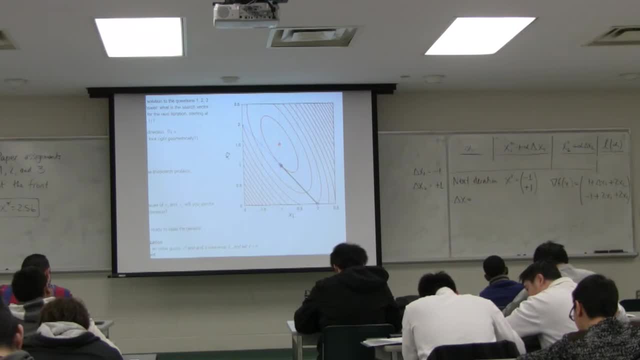 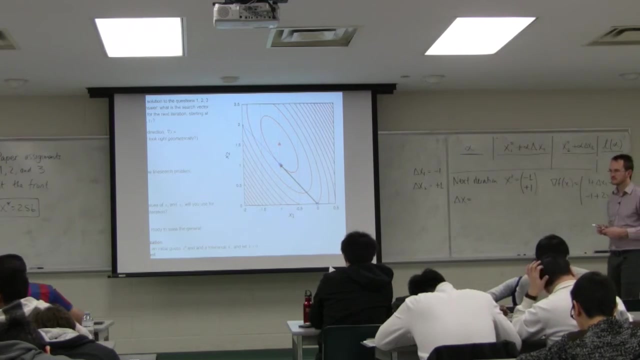 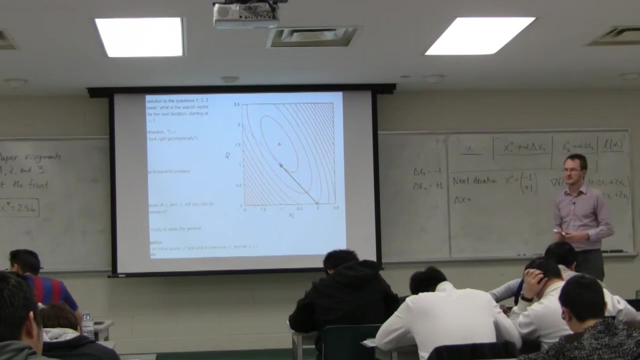 and then go and even solve the line search problem from there. Feel free to work ahead, You can use, You can use, You can use. Everyone get plus one plus one, Okay. so if you sub in there, we're evaluating that function at minus one plus one. 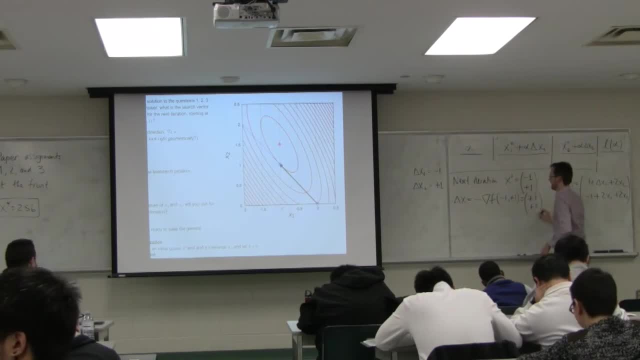 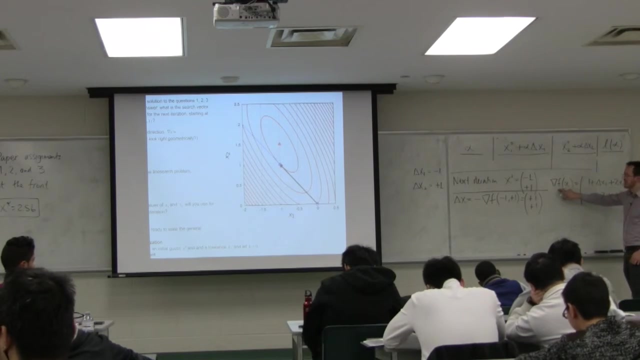 And if you evaluate that, you'll get plus one plus one as your search direction. Okay, so all we're doing is we're evaluating the slope upside down triangle F at our current point. Our current point is minus one, plus one. 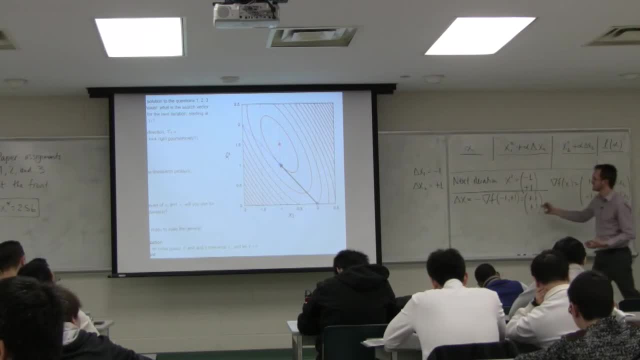 Sub in minus one and plus one at that location. Take the negative of it, because we're trying to minimize and you get plus one plus one Geometrically on that diagram. does that make sense? What is the direction? plus one plus one look like. 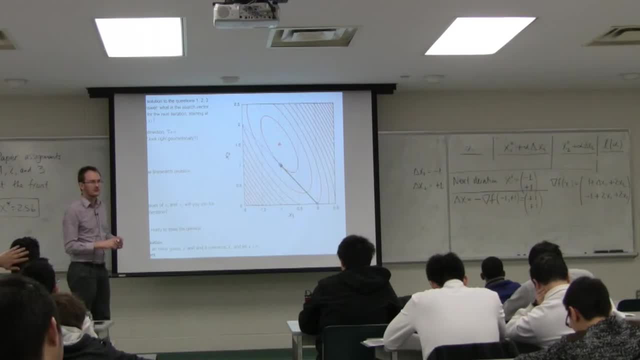 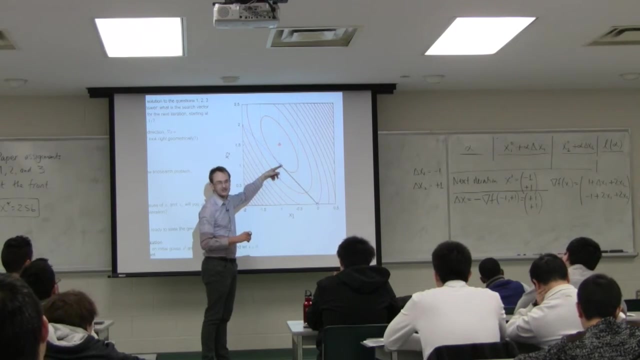 Is that what you expected? What is the direction of steepest descent? We're trying to decrease this function Perpendicular to the contours. What's perpendicular to the contours at this point, At this blue point Plus one, plus one. 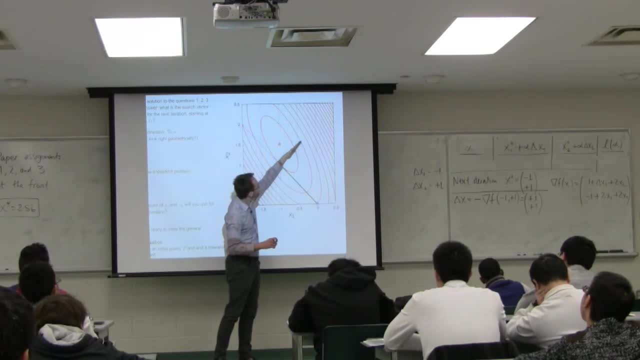 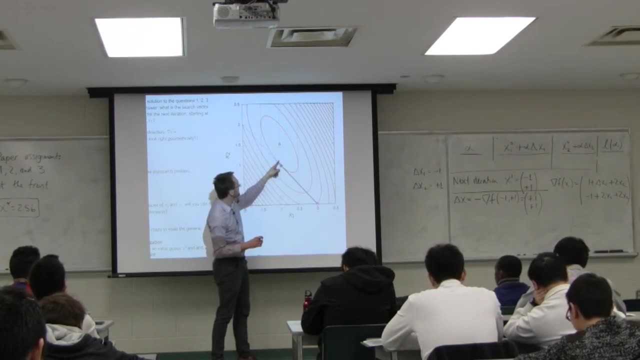 It is in fact that It's more like that, I guess. Yeah, Okay, Forty-five degrees. So that is the search direction. That is the steepest path. If you head that direction, that is not the steepest descent. 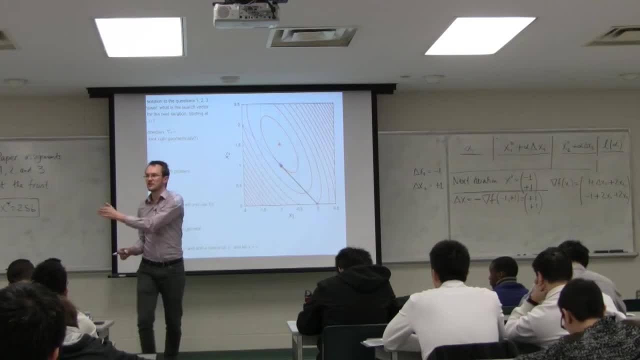 But that's sort of like climbing downhill by walking diagonally. That's the sort of path you take if you're driving a car, So you don't go too fast downhill, But the steepest direction. if you wanted to be tobogganing, you'd be heading that way. 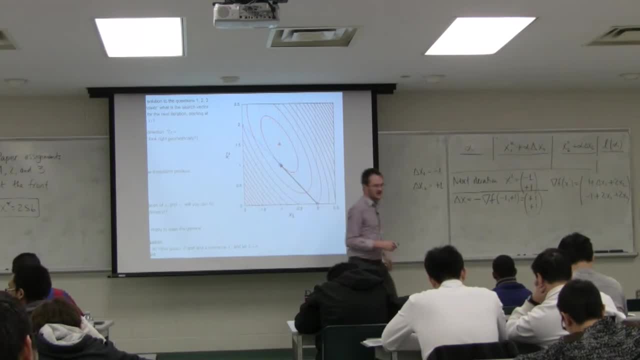 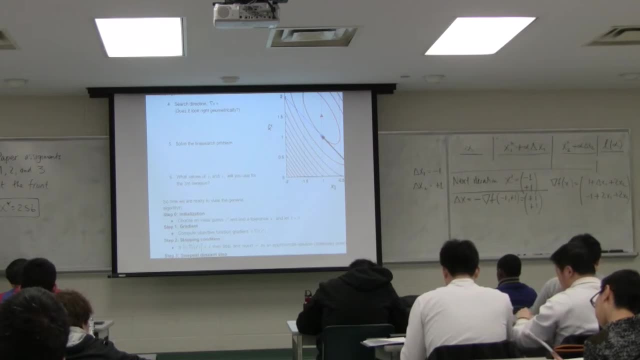 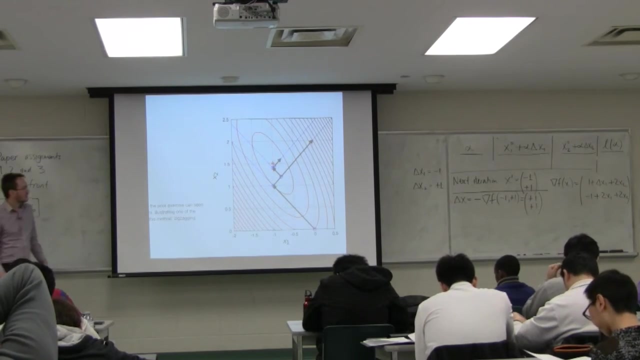 Right Is the steepest direction of descent, So that's actually on the page over. You can flip the page over to see that visually. I've drawn it there for you, Right, Where you notice that we're heading in the plus one plus one direction. 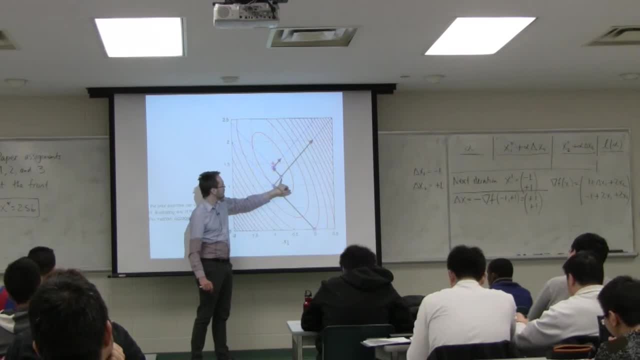 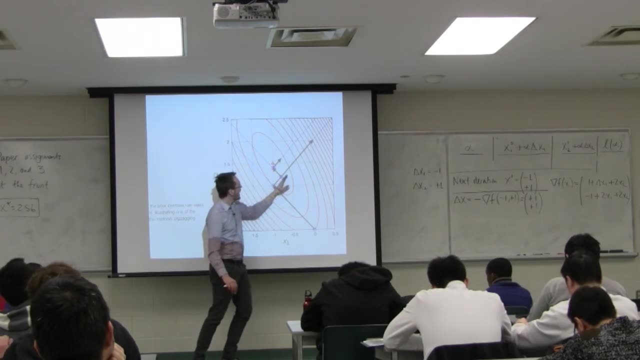 Okay, Now, how far of a step do I take Here? I've shown you the answer. We're going to go to that, Okay. Okay, Next, blue dot. Remember that the computer algorithm doesn't know that. So how far along that direction do we go? 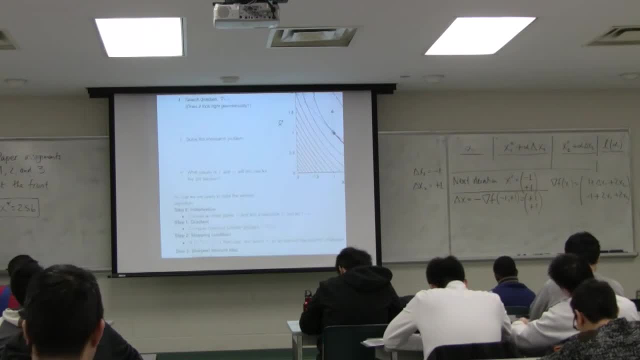 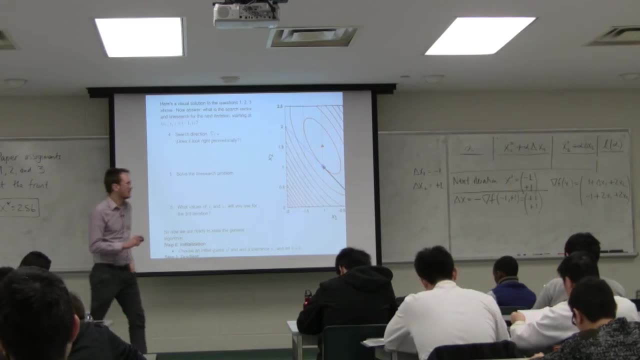 So that's back to the prior page. I've left a little bit of space here for you And that's probably not enough space to solve the line search problem. But let's at least take some points And I'll basically write out the answer here for you so that you can go verify this. 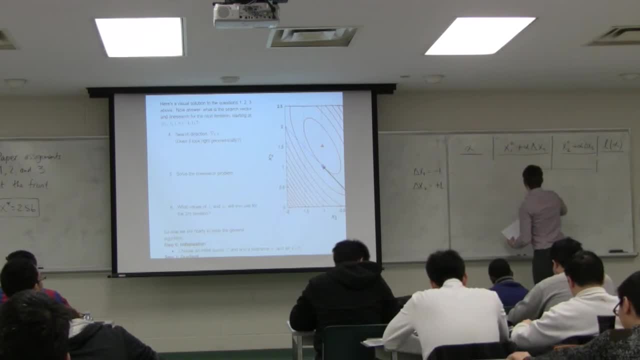 Okay, So what you will do- I suggest you go try this out- is your alpha. then you take an initial alpha at zero, That corresponds to the point minus one plus one your current location, And you'll evaluate the function there as minus one. 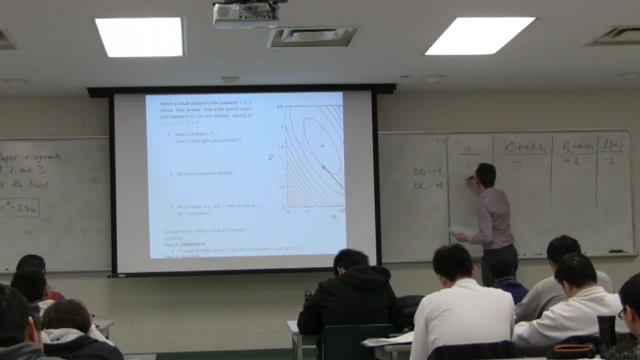 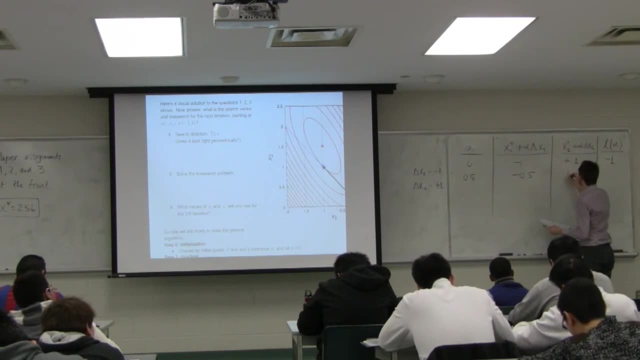 Then you might say: okay, I'm going to take a step of alpha equals 0.5.. If you sub in the values there, you'll land up at the location minus 0.5, 1.5.. And f of minus 0.5, 1.5 is equal to minus 0.75. 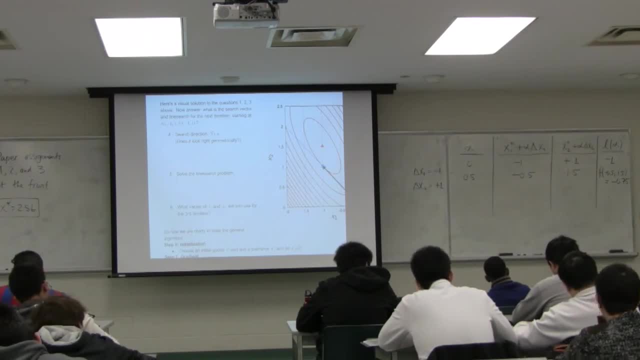 Okay, Now, I know that you're just writing this down and probably not thinking about it, But take a look at what's happened. We've gone too far. We've gone too far. Right, We're at minus one. We're hoping to decrease. 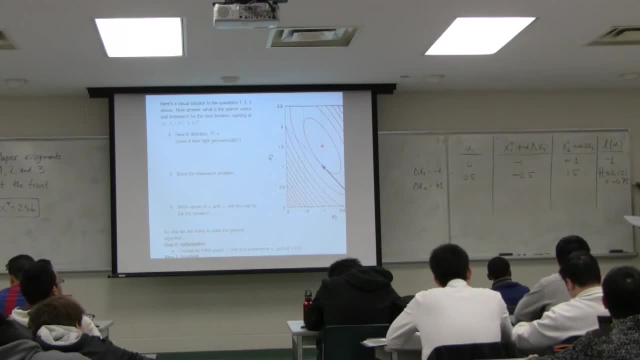 And we've decreased or increased. We've actually increased. We've gone from minus one to minus 0.75.. So we've actually stepped too far. So there's no point in just going to try alpha one, two and further on. 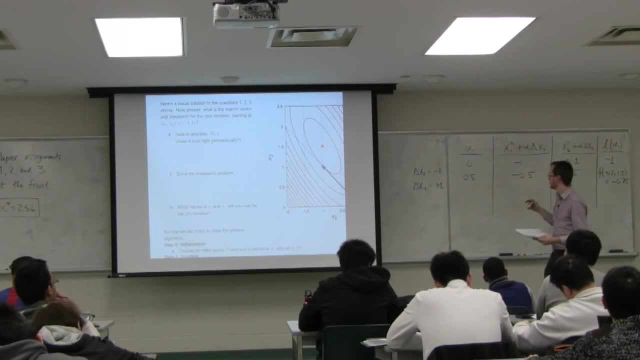 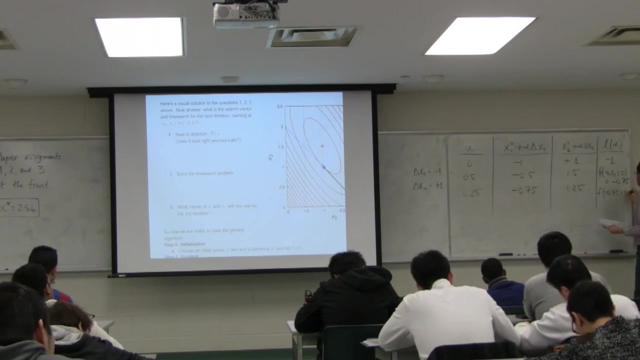 We've actually overstepped the optimum. So let's pull back a bit And let's try 0.25, for example. If you sub in those values, you get minus 0.75.. 1.25. And then f evaluated at minus 0.75,. 1.25 is equal to minus 1.1875.. 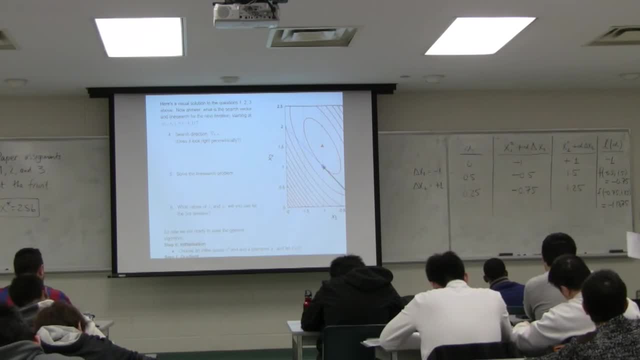 Okay, So which? well, there's your three points to do the quadratic Right. I don't even need to ask you which is your three-point problem. You've got three points. There's a minimum in the middle there And you can go and find the optimum alpha. 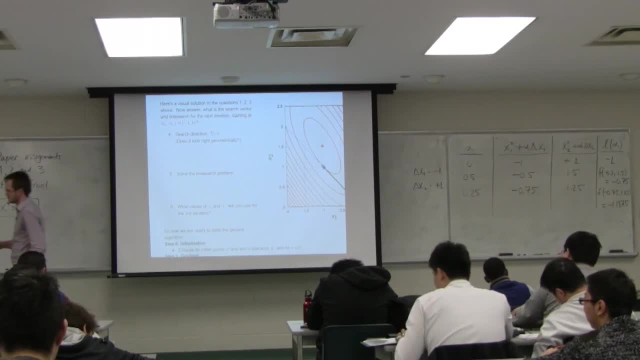 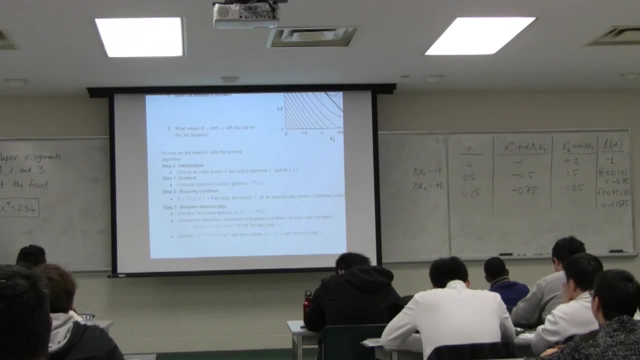 Okay, And that's, That's what the illustration on the page shows you. So you can, You can, You're welcome to work through that, And I've put there, on the bottom of page three, the steps that you would proceed to solve and 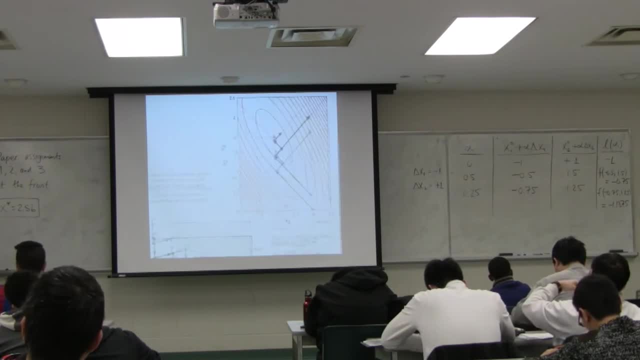 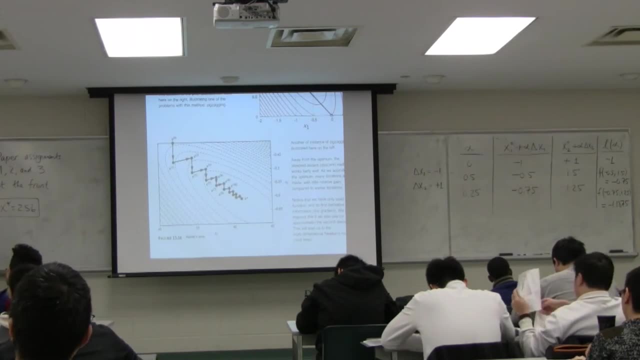 approach the optimum. I know that we're right at the time, So I just want to point out one of the issues that happens with these sorts of methods, And that is what we call zigzagging. It's very typical that these sorts of calculations will proceed. 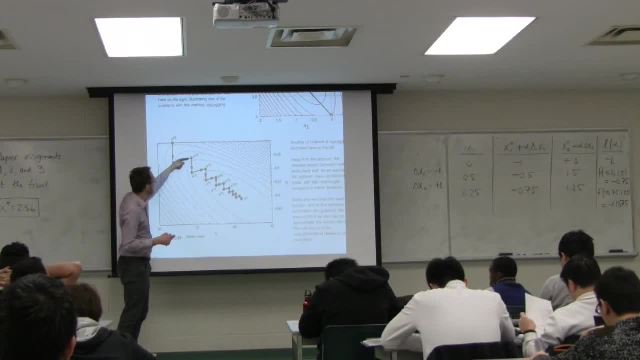 And quite rapidly. It doesn't matter that you're right on the top. If you're right on the bottom You can go and find the optimum. Notice here that every time we're going perpendicular to the contours. But those last few iterations are. 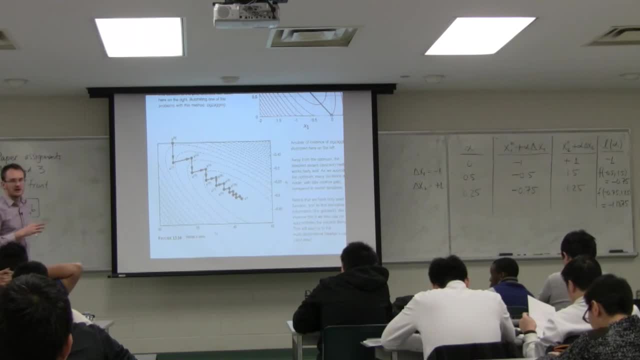 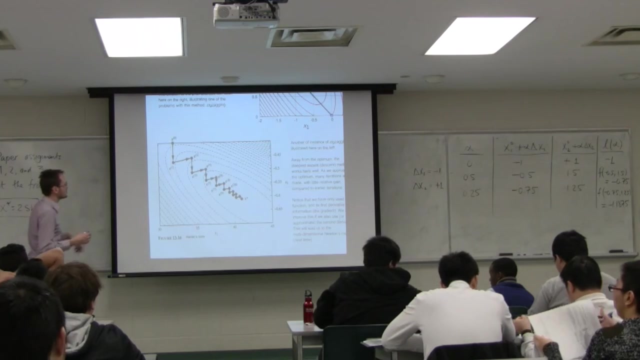 Make very, very slow progress. Okay, So what we're going to do is in next class, is Well? next, After the break is: look at Newton's method to try and get past those slow convergence steps. Okay, Newton's method will get to the optimum in about two or three iterations here. 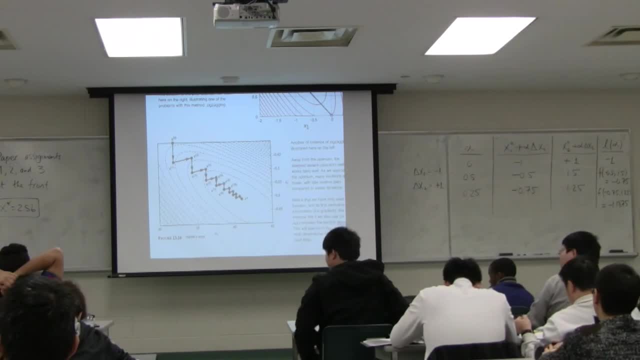 So I'm going to show you the bottom. So that's where we'll leave it. That's also where the midterm is up till on Monday. I'm debating to have a class on Monday. I'm not sure if it's a good idea to be teaching you stuff on Monday.